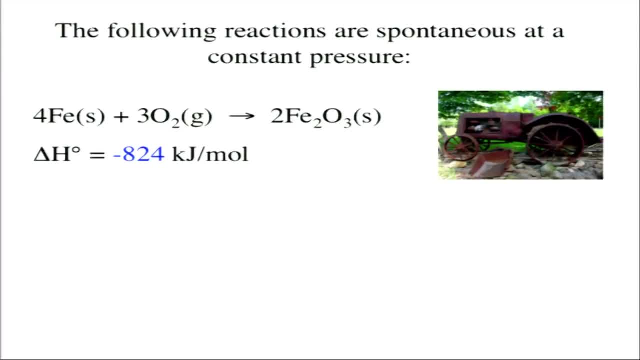 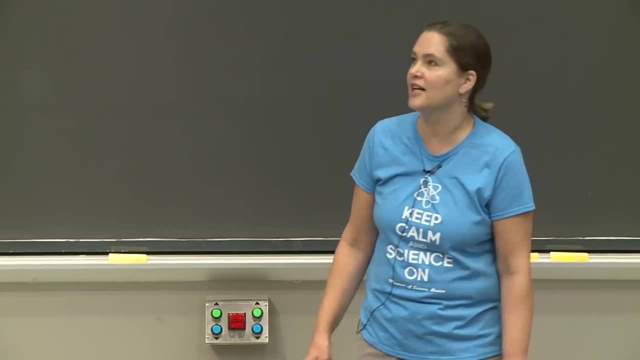 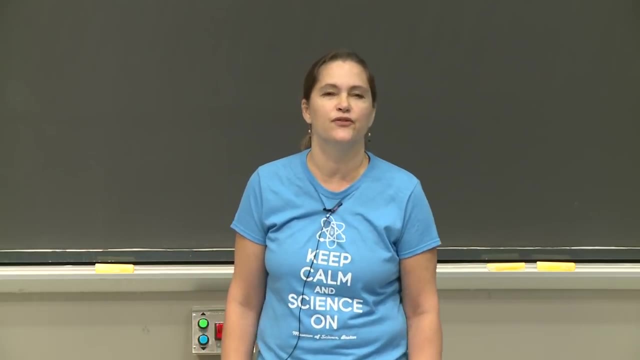 Iron plus oxygen. And what is this in layman's term? an example of Rust? Rust, yes, And many of you are probably aware of this. Rust is a spontaneous process. It's something that people try to do something about. You don't want your car to rust. 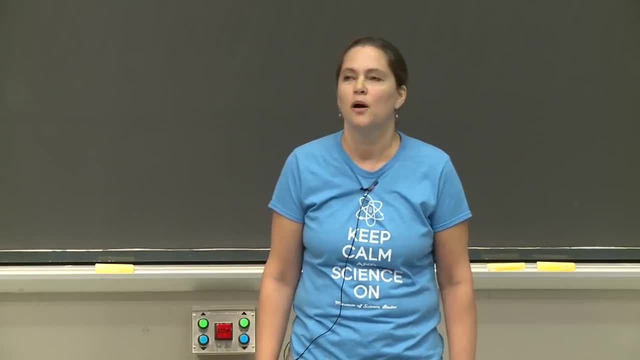 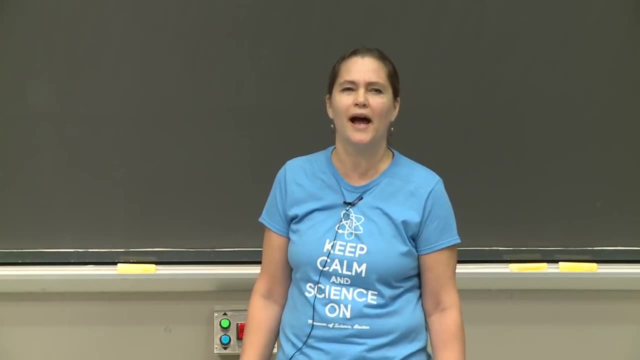 If you're new to New England and you're from a part of the country that doesn't get so cold, you may not have. you look at people's cars and you're like, wow, look at all that rust all over them. Yes, rust happens, especially in New England. 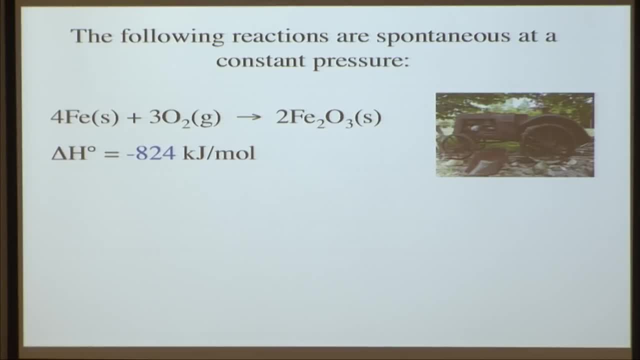 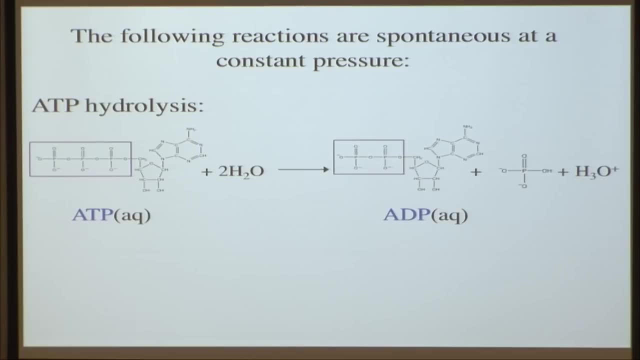 And delta H here is negative. Is this endothermic or exothermic? Exothermic Minus 824.. OK, here is another spontaneous process. This molecule is ATP And it will hydrolyze, which means react with water. 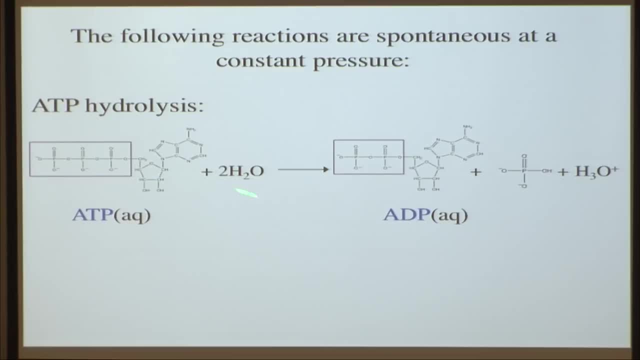 forming ADP. So ATP is triphosphate, ADP is diphosphate, So one of the phosphates- and here's the other- phosphate comes off, It hydrolyzes off, And this is a spontaneous process. We also have a delta H naught of minus 24 kilojoules per mole. 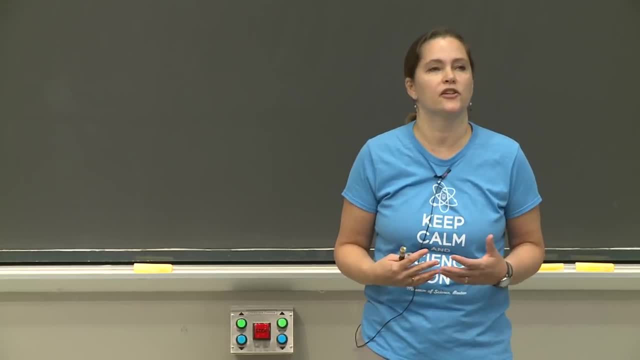 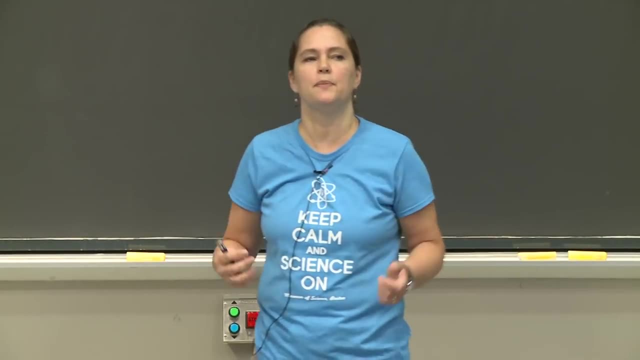 And remember, when we oxidize glucose in our body, we store that energy in ATP And we want that ATP to be around And then, when we break ATP apart, it releases the energy. So this is a very important biological process And you have a negative value. 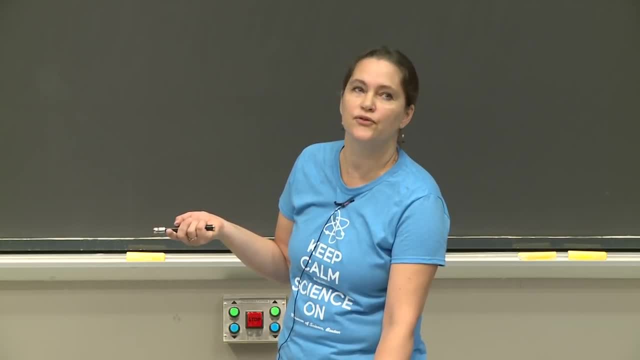 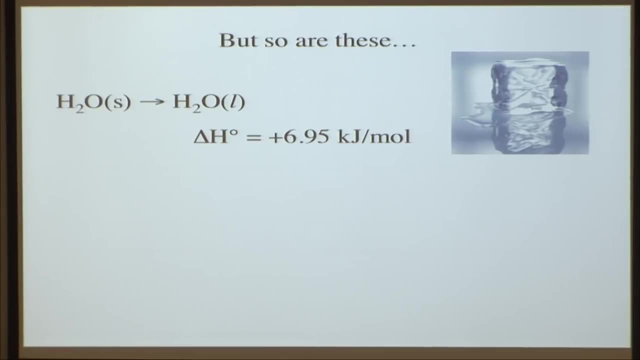 So you have an exothermic reaction. But there's a few other examples of spontaneous reactions. One of them is this one, And we've probably all experienced this: If you're from New England, you've seen snow melt. So you've seen ice melt solid to liquid. 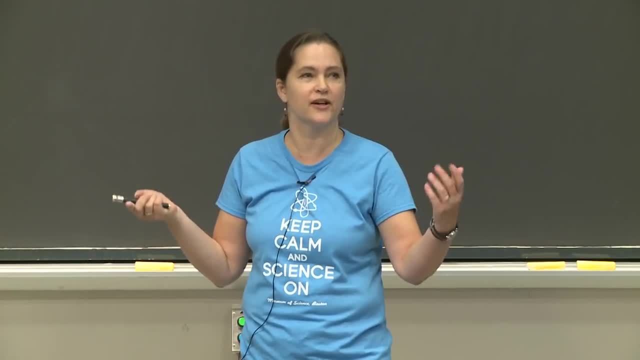 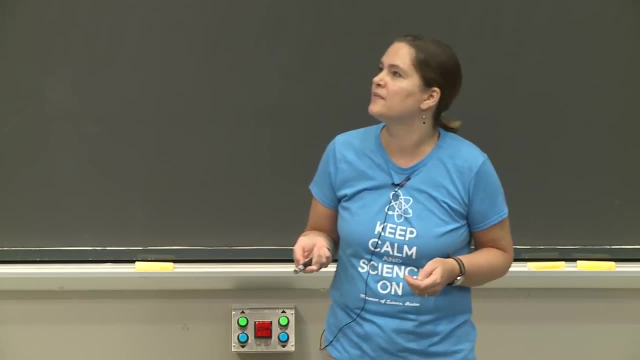 If you're from a hot part of the world, you probably had ice cubes in your nice refreshing drink, with maybe a little umbrella on the top. Anyway, everyone, I think, has seen ice melt. OK, But here delta H naught is a positive value. 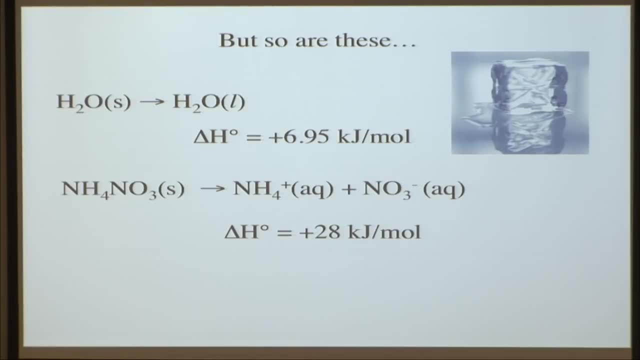 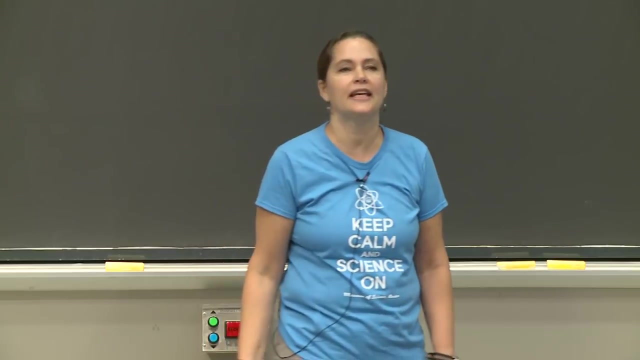 It's endothermic. Also, if you have ammonium nitrate, this will just come apart in a spontaneous reaction. Delta H here is plus 28 kilojoules per mole. So is delta H the key to spontaneity. 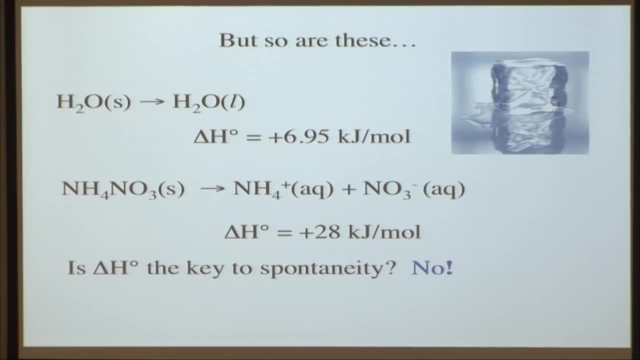 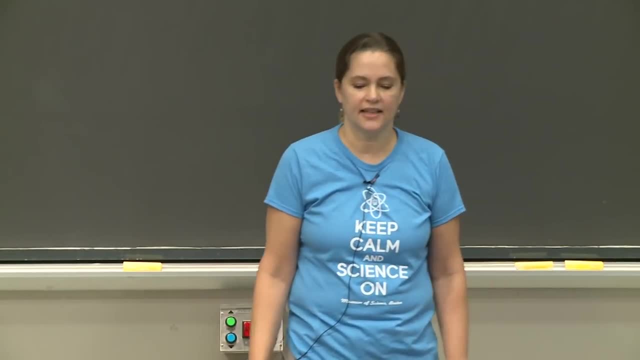 It is not, It plays into it, But it's not. It's not, It plays into it, But it's not. But it is not the determining factor. So if delta H naught is not the key to spontaneity, what is? 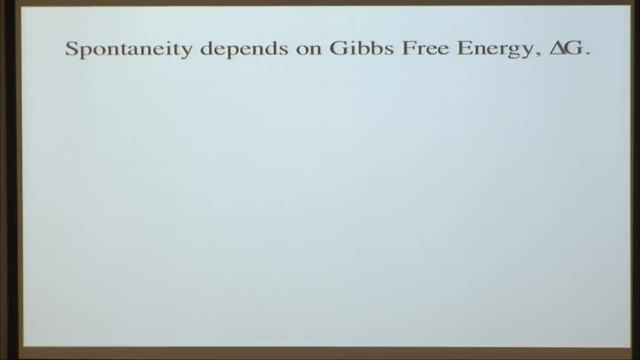 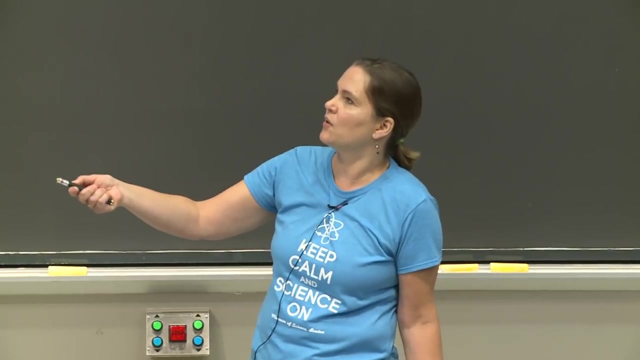 It is free energy. yes, Particularly Gibbs free energy or delta G, And I'm really happy they decided to add the Gibbs free energy, because another thing of energy would be a lot. So having this free energy, Having an abbreviation of G, I think is a good thing. 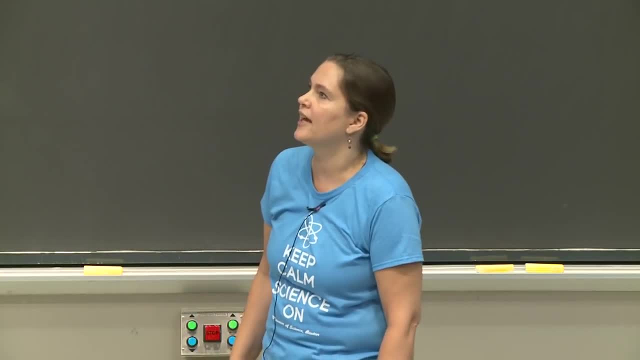 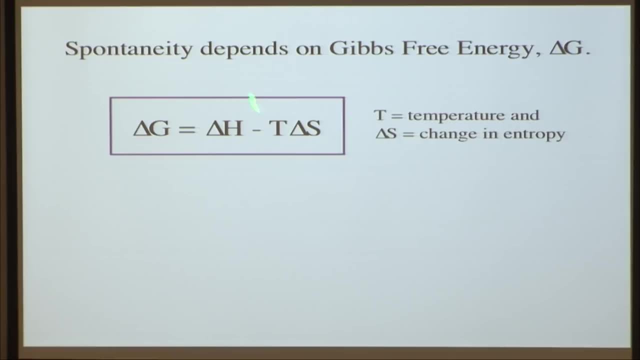 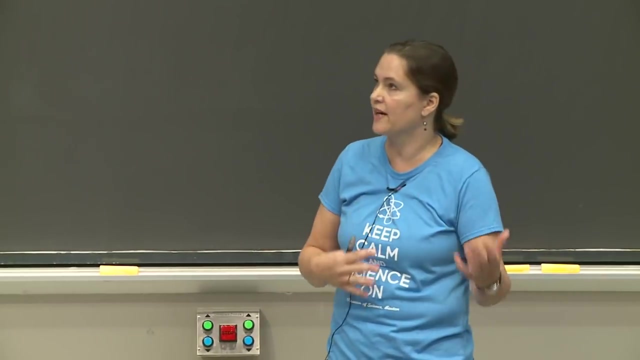 So Gibbs free energy. So Gibbs free energy depends on delta H, But it also depends on another term, which is T, delta S- temperature and delta S- change in entropy. So delta G is the predictor of whether a reaction will go forward in the forward direction. 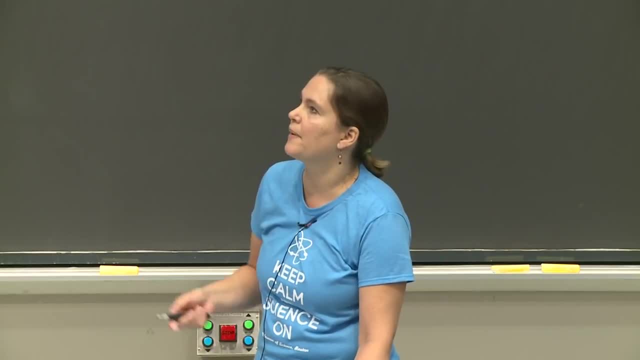 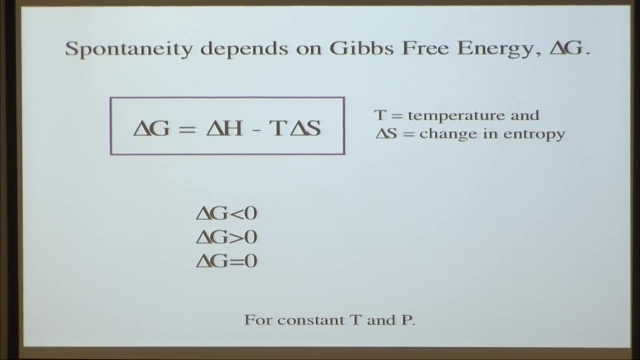 in a spontaneous fashion or not. So let's just think about the sign of delta G and what it means. So again, at constant temperature and pressure, here delta G less than 0, negative delta G. is that spontaneous or not Spontaneous? 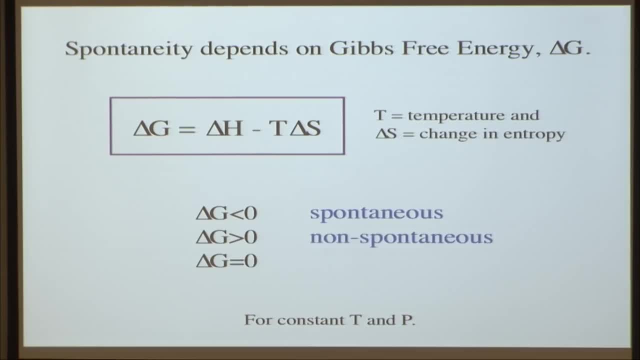 Positive. delta G is not spontaneous, non-spontaneous, And delta G equals 0. It's one of the obvious, It's one of the other things that I am very fond of, which is equilibrium. So delta G indicates whether something is spontaneous or not. 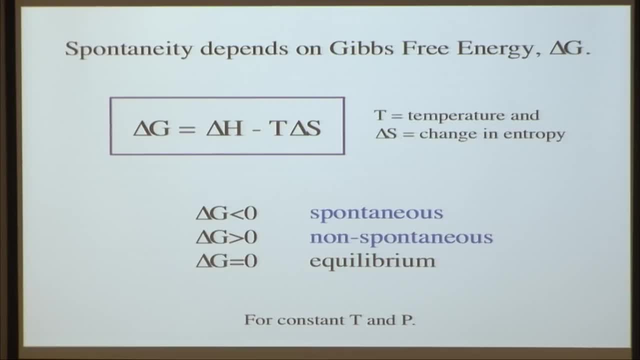 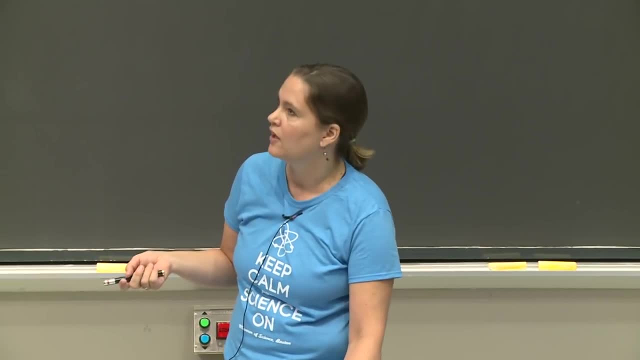 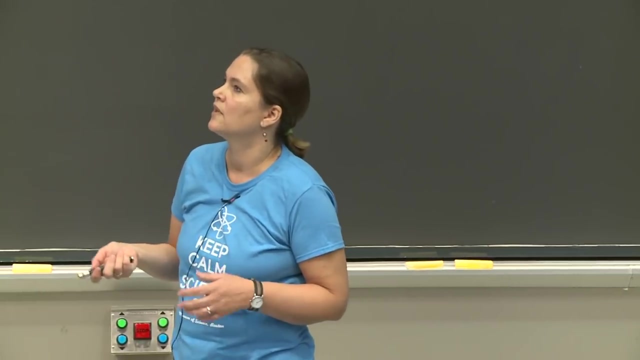 Negative value spontaneous in the forward direction. Positive value, not spontaneous in the forward direction. And equilibrium, the thing we all try to reach in our lives. So let's look at an example and calculate what delta G is going to be. So we saw this equation already. 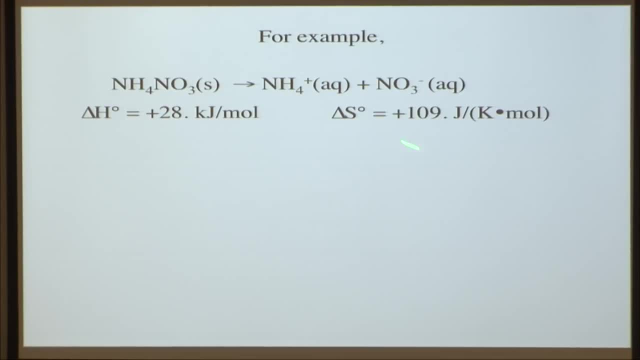 We have a positive delta H0. And now I'm telling you that delta S0 is also a positive value, So we can use this equation, And this is really one of the most important equations in chemistry. Figuring out this equation was really a crowning achievement. 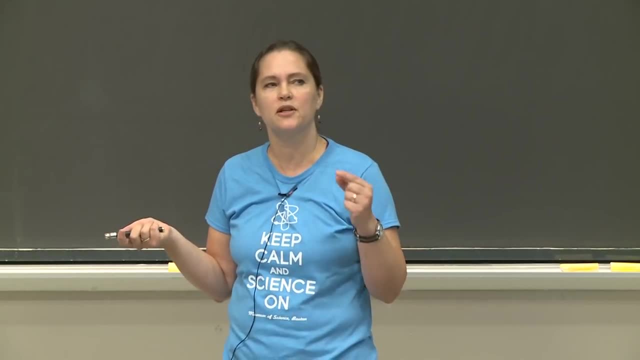 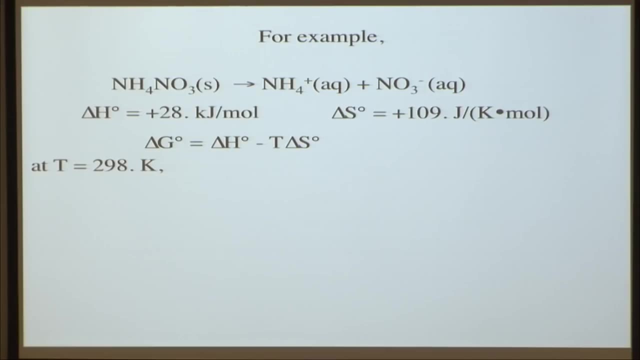 And you'll be using it a lot, not just in this unit, but pretty much in every unit. from now on You will be using this equation, All right. So room temperature, pretty much we're not doing. Occasionally we'll do something, not at room temperature. 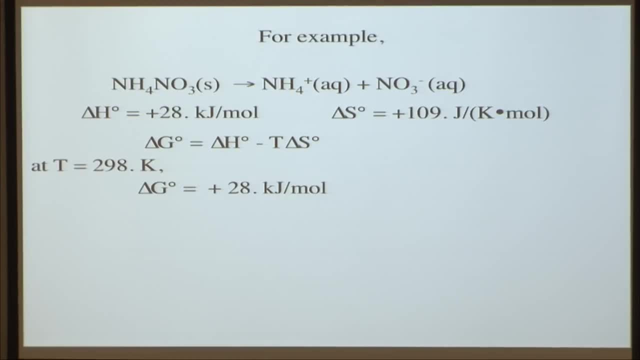 but we like room temperature And we like it in Kelvin, So delta G0, so we plug in our delta H value. So it's going to equal delta H minus the temperature, And if the temperature isn't given in a problem, you can assume that it's 298.. 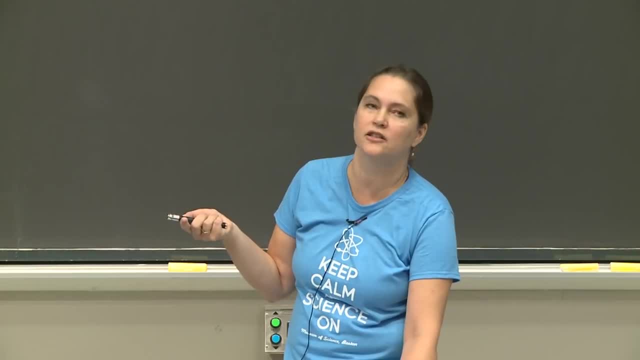 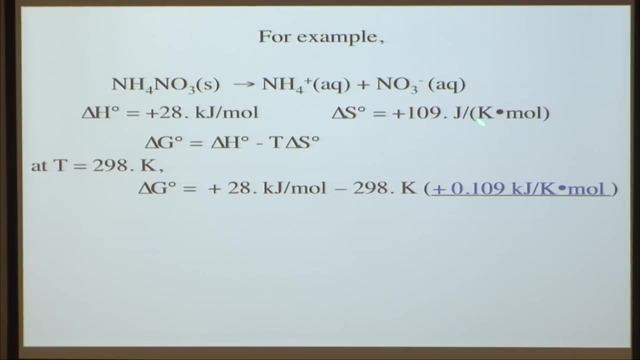 And now we need to plug in delta S. But I left a blank here to make a point, Which is that delta S's are almost always given in joules per Kelvin per mole, But everything else is given in kilojoules. So you want to make sure you convert your units. 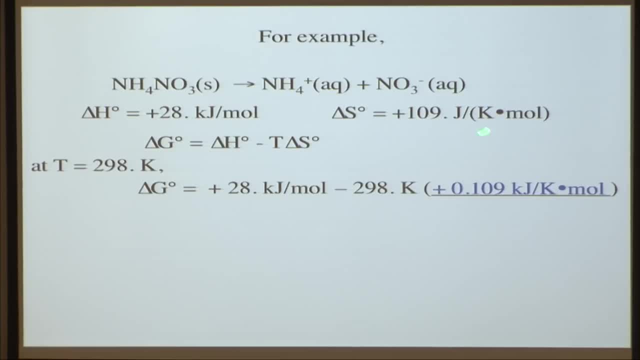 or you're going to come up with very funky answers at the end. So, from joules to kilojoules, so now plus 0.109 kilojoules per Kelvin per mole, And we can do this out now, So we have plus 28.. 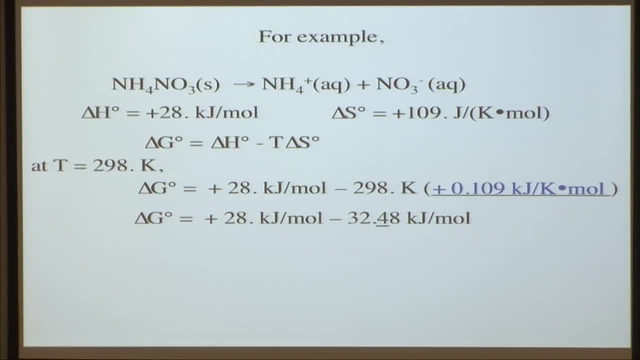 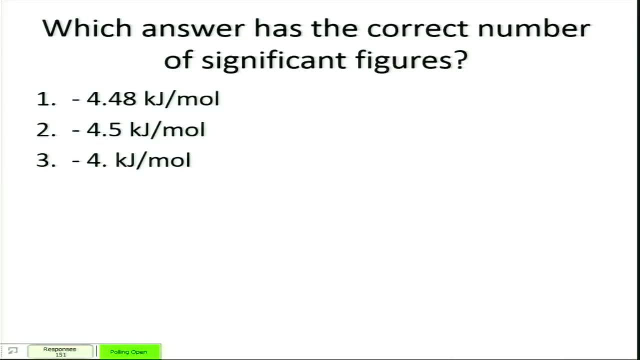 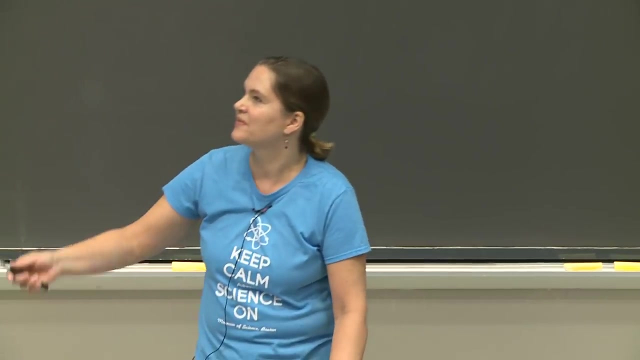 Minus 32.48.. And why don't you tell me how many significant figures this answer has? OK, 10 more seconds, OK. so at least some people got it right. We've identified once again a weakness. So rules of adding and subtracting. 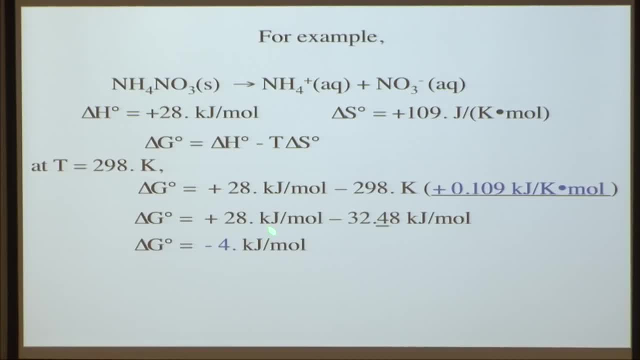 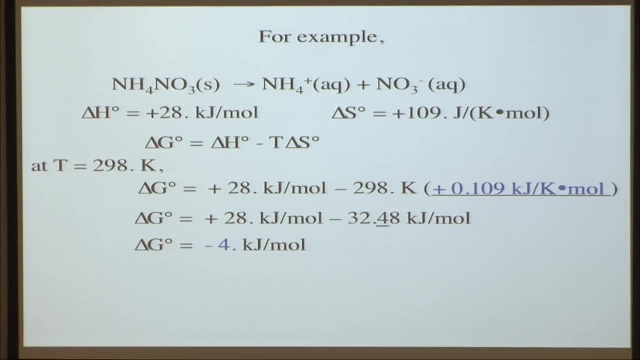 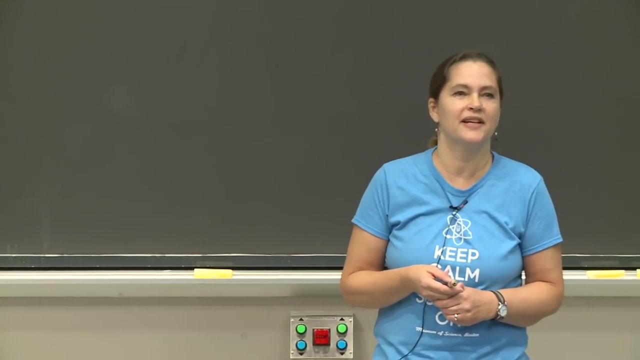 So we're just left with 4.. So when we're doing multiplication or division we consider the total number of significant figures. But with addition and subtraction you've got to pay attention to where the decimal point is. And when we get into the next unit there are logs. 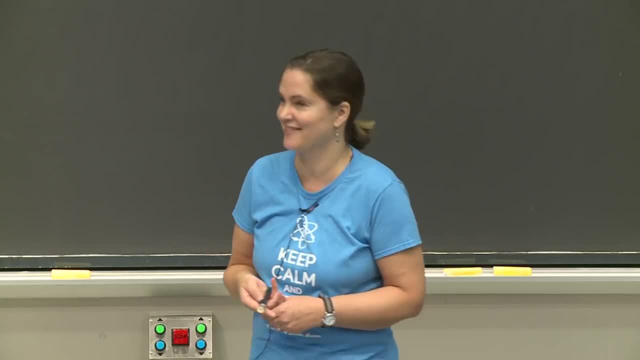 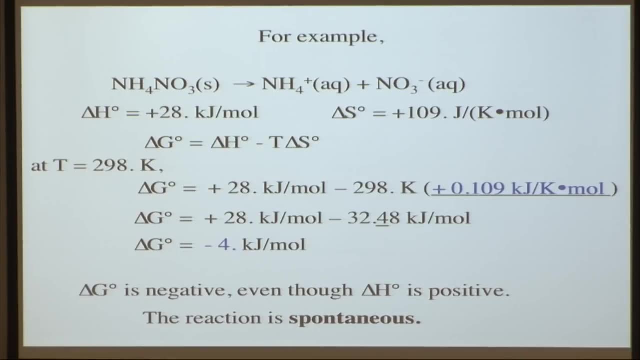 And those have special rules of significant figures. So we're going to look at these in a minute, But before we do that I want to give you a little bit of information about the delta H. Yes, very exciting, All right. so delta G0 is negative here. 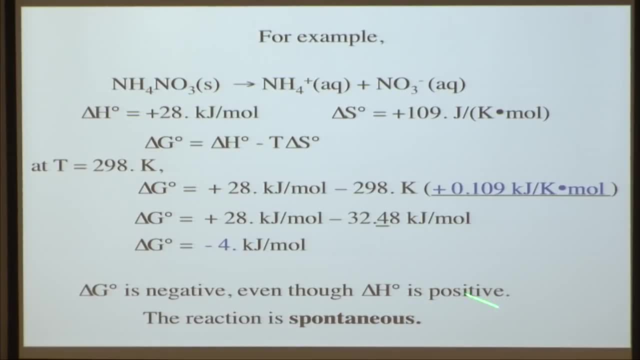 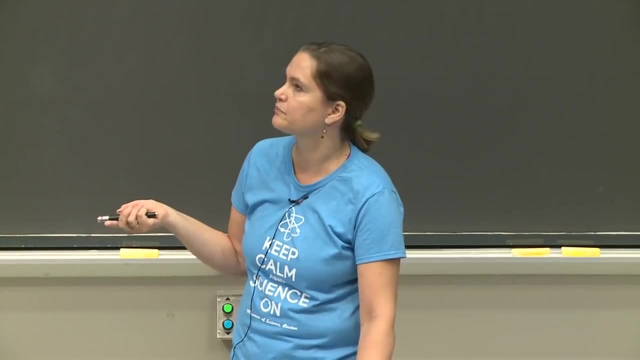 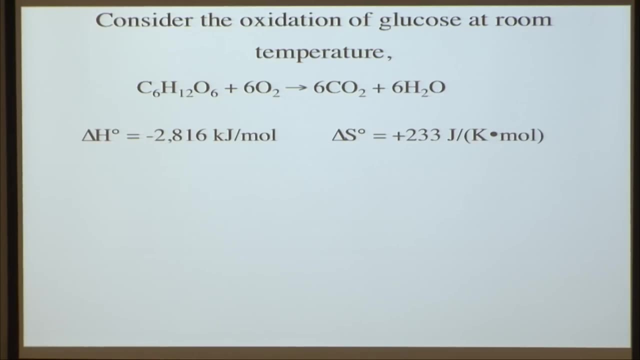 although delta H is positive. So this reaction is spontaneous. It's not hugely, It's a pretty small number, But still it's spontaneous All right. so let's consider our friend over here that we've been talking about glucose being oxidized to CO2. 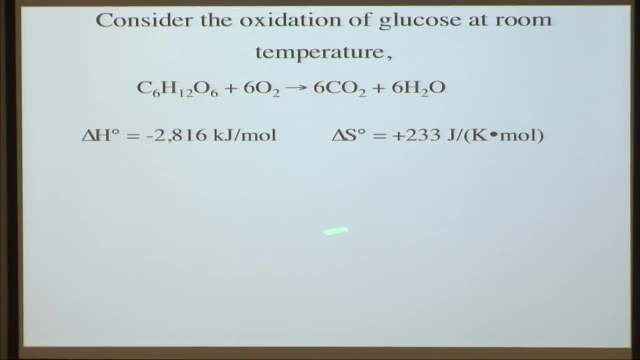 and water. You practically should have the delta H memorized for that at this point. Now I'm telling you what the delta S0 is, And it's positive 233 joules per Kelvin per mole And we can plug this into our equation. 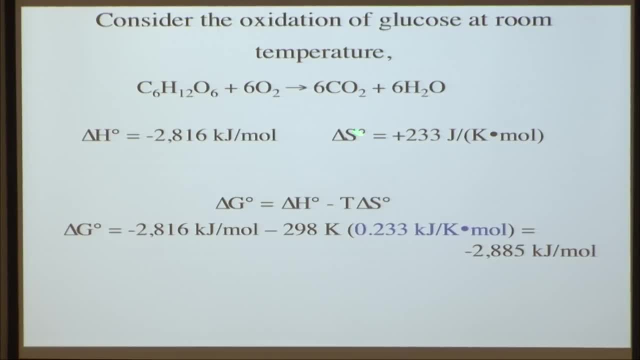 to calculate a delta G0, again remembering to convert joules to kilojoules to do this. And so now we see that it has a very negative delta G0 here, minus 2,000.. Minus 2,000.. 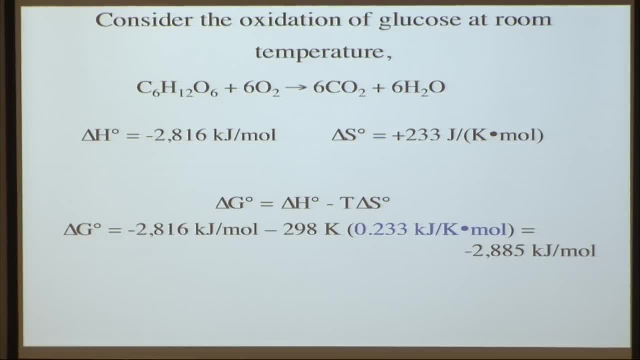 It's 2,885 kilojoules per mole at room temperature. So at room temperature this reaction is spontaneous but slow. We saw that with the candies that had glucose in it. We opened them up and no water or CO2. 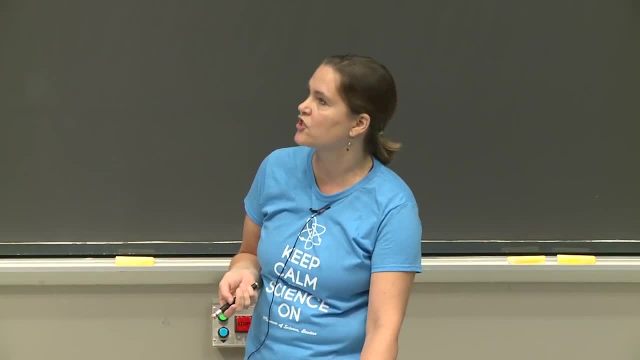 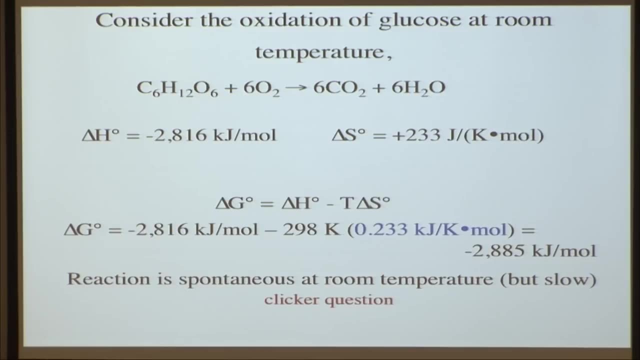 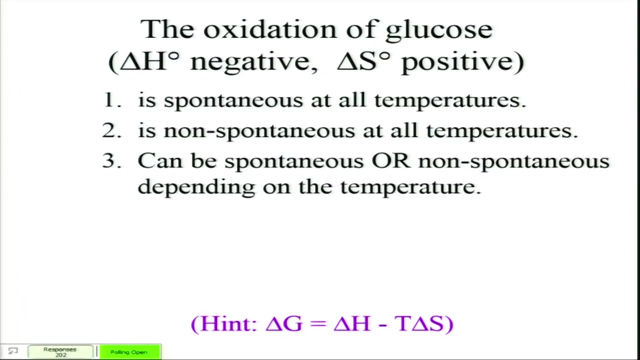 were obviously being liberated in this reaction because it is slow. And now a clicker question. I want you to tell me whether it would be spontaneous at different temperatures or not. OK, 10 more seconds. Yep, So it is spontaneous at all temperatures. 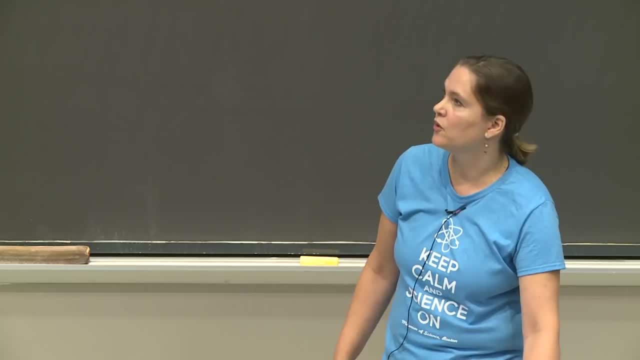 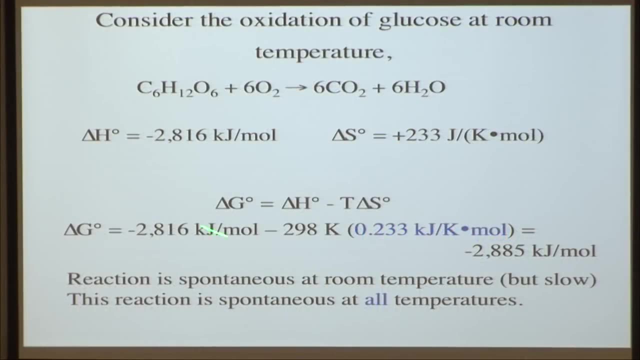 Not all reactions are, but this one is. So if we go back here, the reaction's spontaneous at all temperatures, And that's because to be spontaneous, you want a delta G that's negative. If delta H is negative and delta S is positive, then you'll. 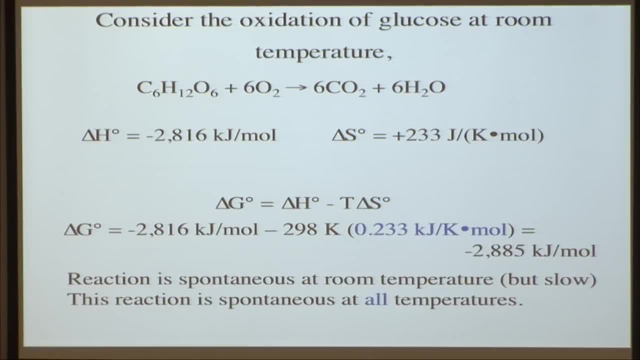 have a negative minus a negative, So it doesn't matter what temperature is- This will always yield a negative delta G0.. So other reactions that might not be the case, But if you have negative delta H and a positive delta S, it will be spontaneous. 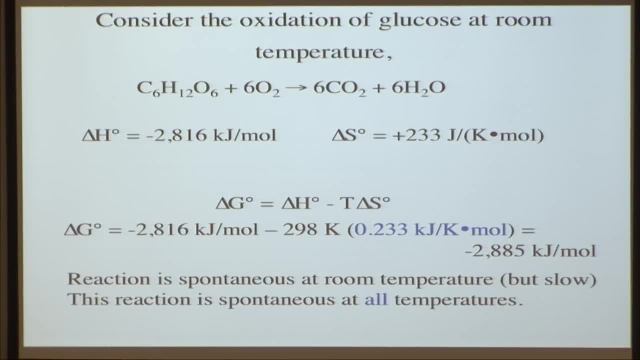 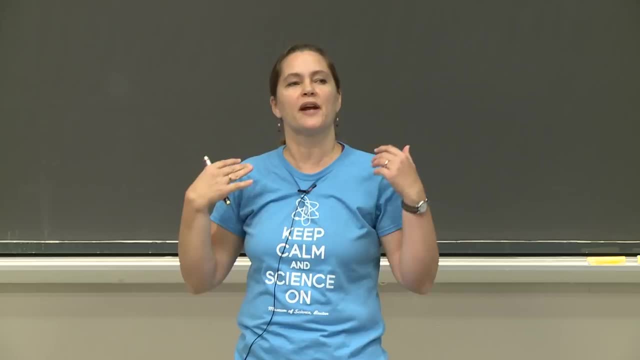 So negative delta H again, exothermic heat release And a positive entropy is a favorable thing. Entropy is always increasing, So if this reaction has increased increase in entropy, it'll be much more likely to be spontaneous. All right, so. 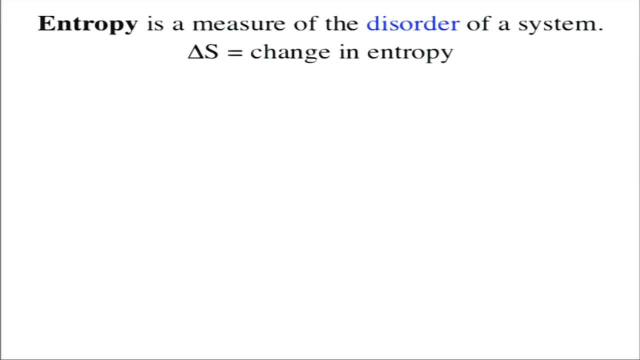 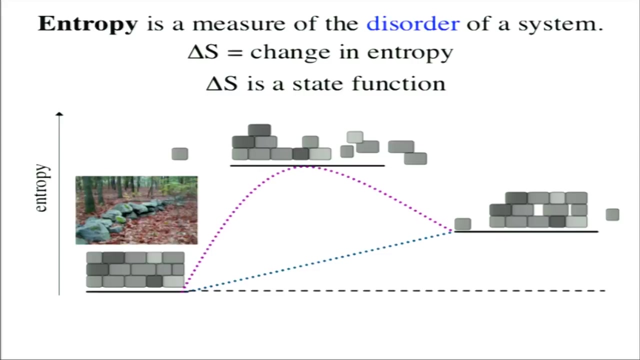 let's talk about entropy. So entropy is a measure of disorder of a system. Delta S is the change in entropy And Delta S again is a state function. So one example of entropy in New England are these stone walls that do not look absolutely. 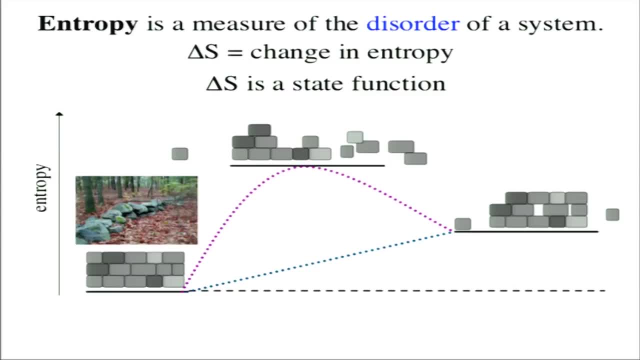 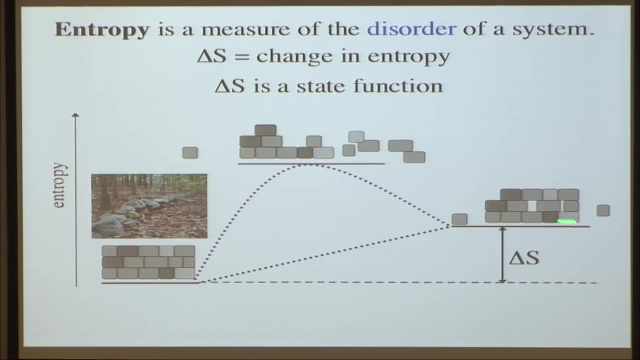 beautiful. They're often stones falling everywhere And it doesn't matter if these stone walls were probably built in 1600s or 1700s in New England, fell totally apart and were rebuilt Now. we just care about how the wall is compared to the way it started. So Delta S again is a state function. It. 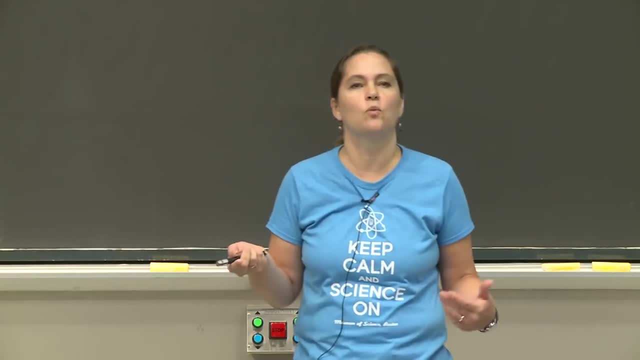 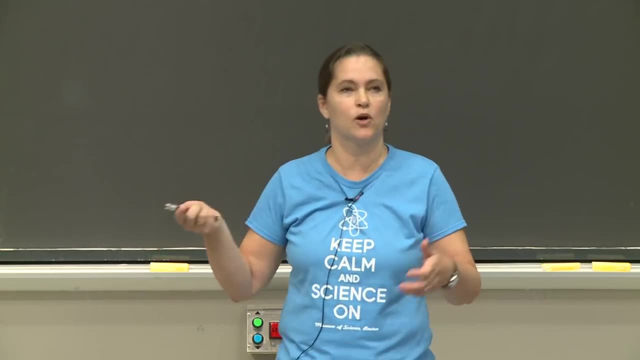 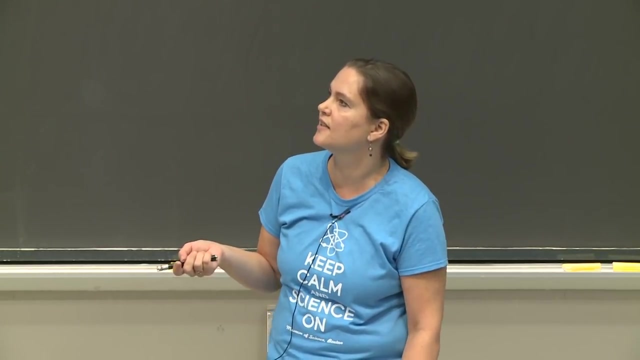 doesn't depend on path. And so if you get out and walk around and go like on the minute man trail and say some of the historical sites where Paul Revere rode his horse, along a lot of stone walls, There's a New England poet who writes about this, Robert Frost, and he said something. 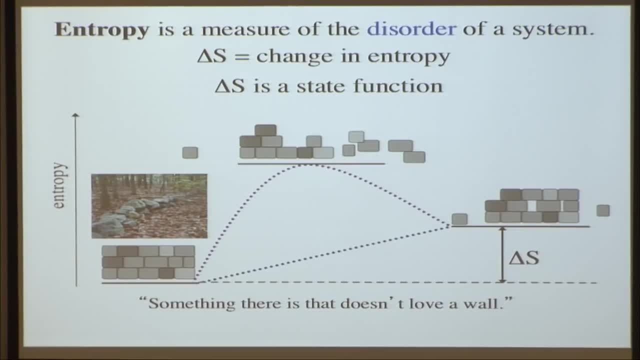 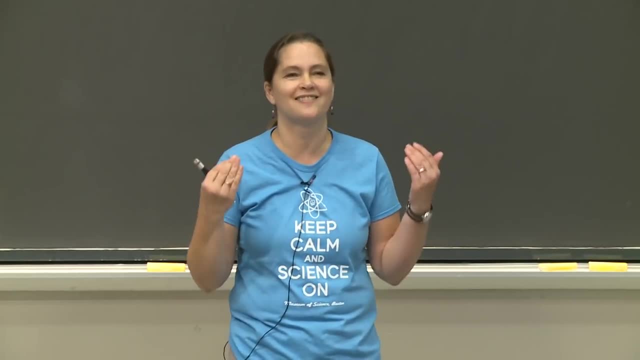 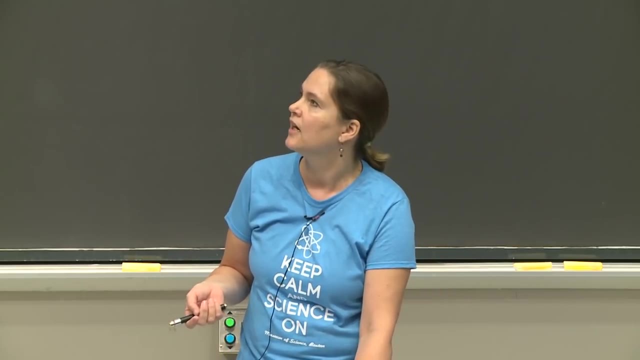 there is that doesn't love a wall and that something is entropy. Entropy does not love a wall. Entropy does not like order. Another example: those of you who are learning more about me as a person know that I am a fan of dogs. 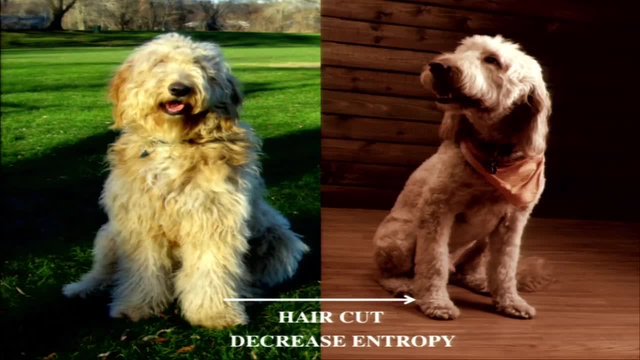 This is my dog Shep. Shep does not like going to the groomers, does not like it, And I think that this is because he's been at my office hours and he knows that increasing entropy is favorable, decreasing entropy is not. 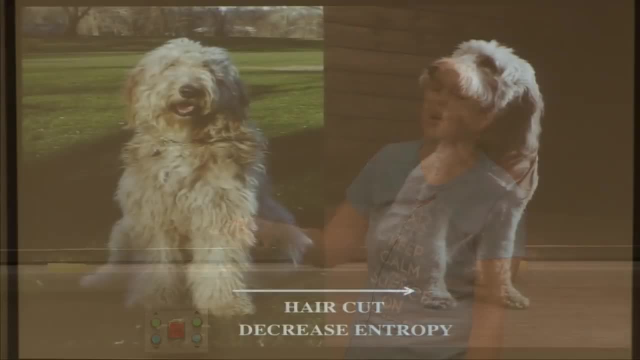 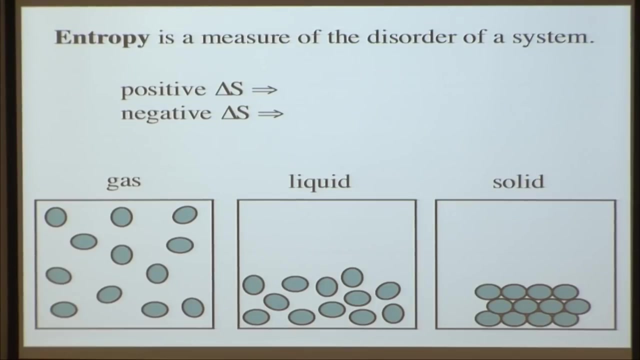 And he says: you know, really, this violates the laws of thermodynamics. What you're doing, You're doing to me and you should cease and desist. But anyway, he still gets haircuts, All right. So entropy again is this measure of disorder of a system? 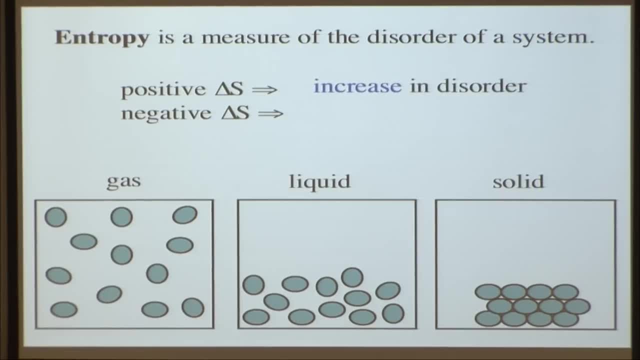 You have a positive delta S which is going to be an increase in disorder, And a negative delta S is going to be a decrease in disorder, And a disorder can be. you can be thinking about this as internal degrees of friction. You can be thinking about this as degrees of freedom in your molecule. 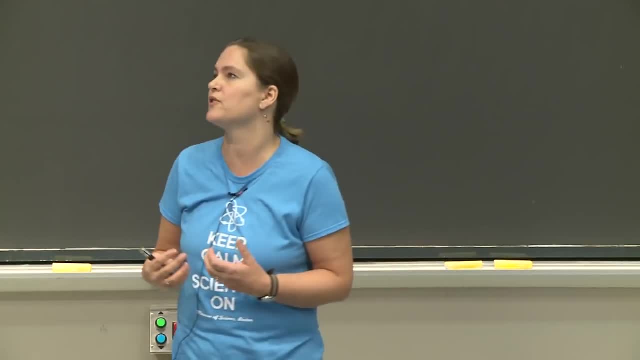 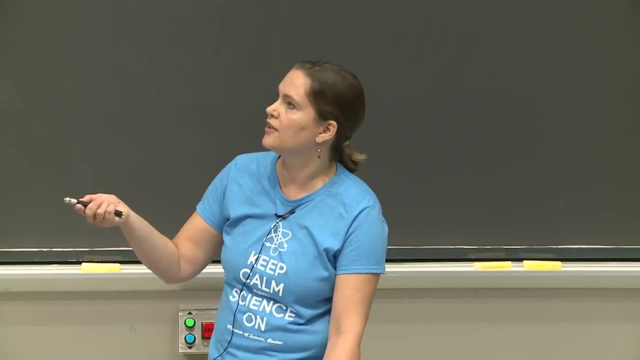 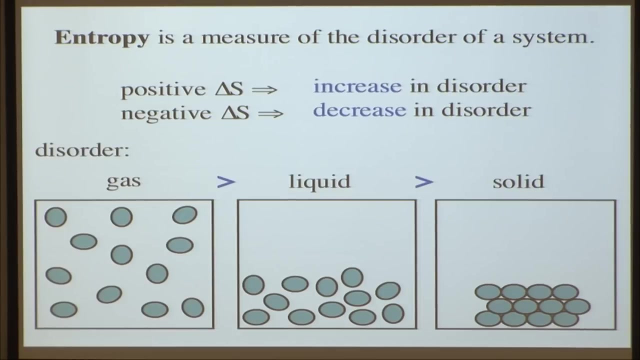 You can be thinking about this as vibrations- All sorts of different things- can lead to increase or decrease in entropy, But we often think about changes in entropy depending on if the reaction is changing in phase. So gas molecules have greater disorder than liquid And liquid has greater disorder than solids. 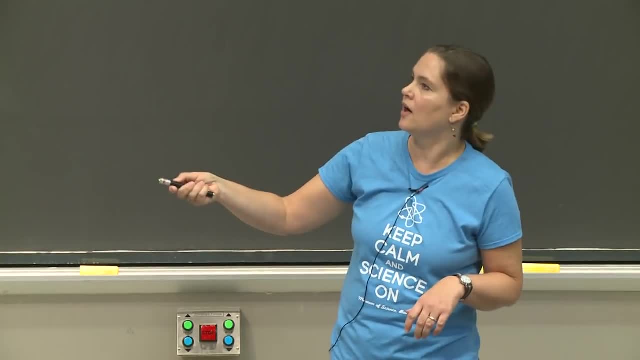 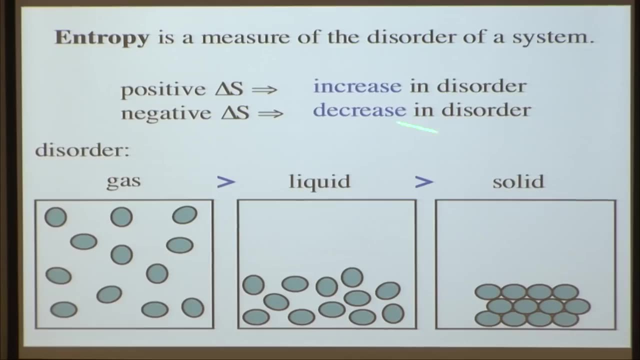 And so a solid has all its molecules lying down And liquid can move around a little bit more, But gas really can spread all out. So, in terms of entropy and changes in entropy, we can think about the phase change that's happening and even predict if something is going to be an increase in entropy or not. 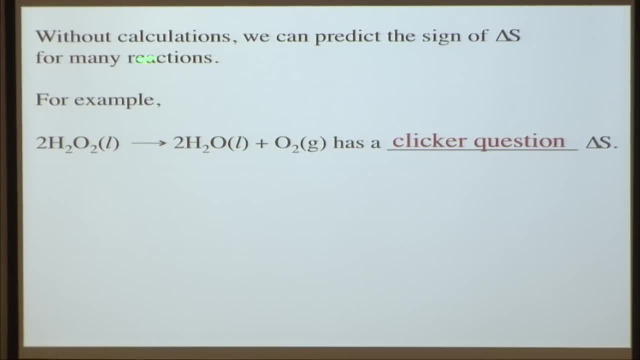 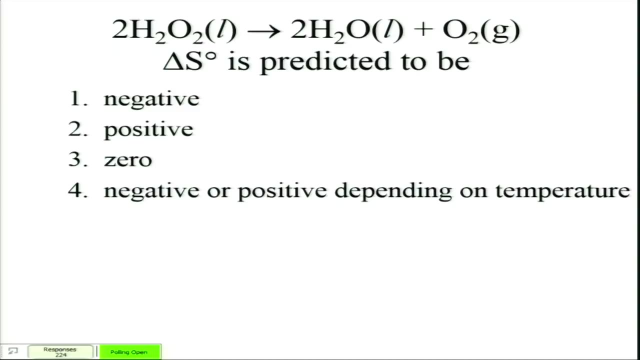 So let's just look at one example. So, without a calculation, predict the sign of delta S? And this is a clicker question. OK, All right, And all right. All right, Let's just take 10 more seconds and can our demo TAs come down? 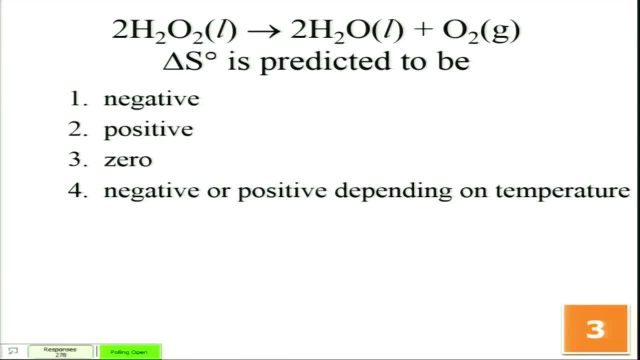 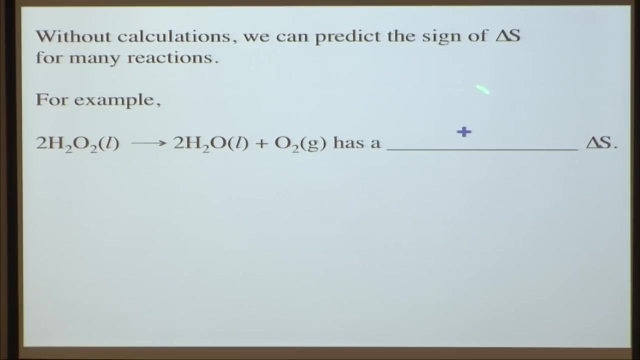 All right, OK, OK, OK, Yep, Good. So you predicted positive, which is the correct answer. And so here we're, going from a liquid to a liquid and a gas, And so going to the gas. that'll increase the disorder. 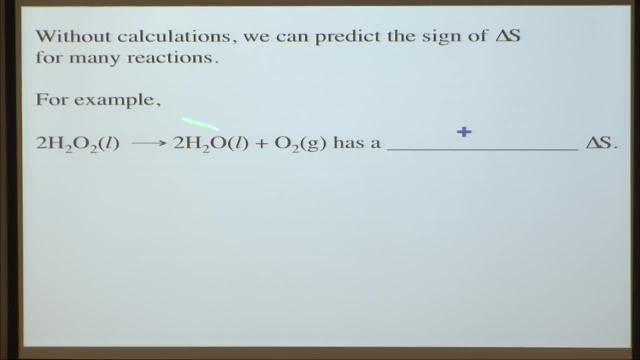 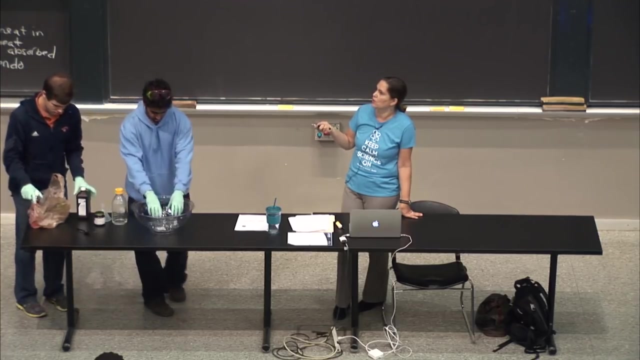 of the system. so delta S will be positive. So now we're actually going to do a demo of this particular reaction And so we have hydrogen peroxide which can just be bought at a CVS or a local drugstore, And it will go to liquid water and also oxygen gas, And so how do you see? 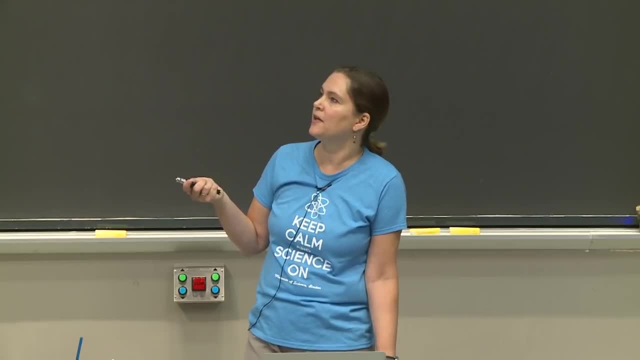 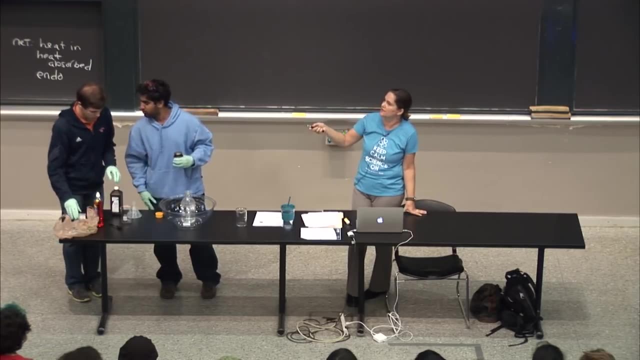 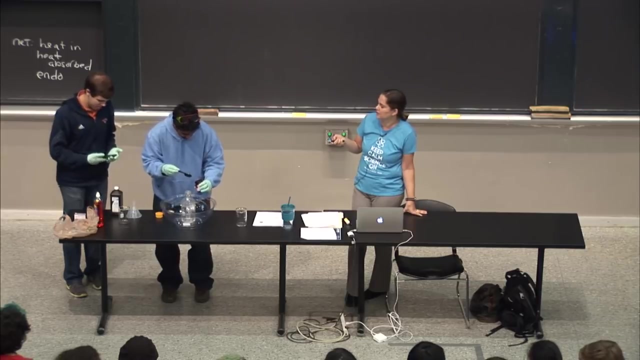 a gas, And you can see it by putting it in with soap bubbles. So as bubbles of oxygen form, the soap bubbles will bubble out, and so you can see it. And you can also add some kind of food color, And we have yeast as a catalyst to make it go a little bit faster. So let's see if we can. 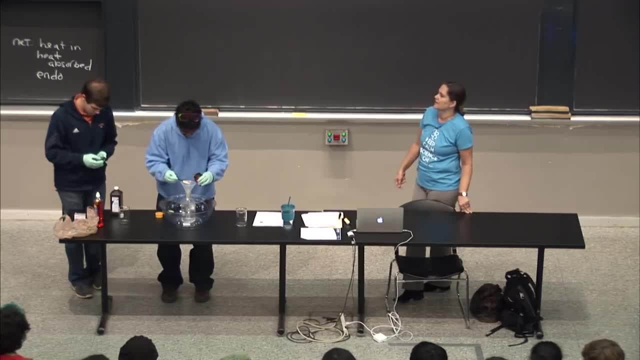 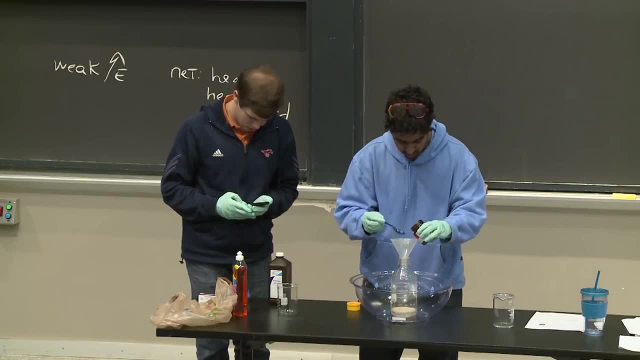 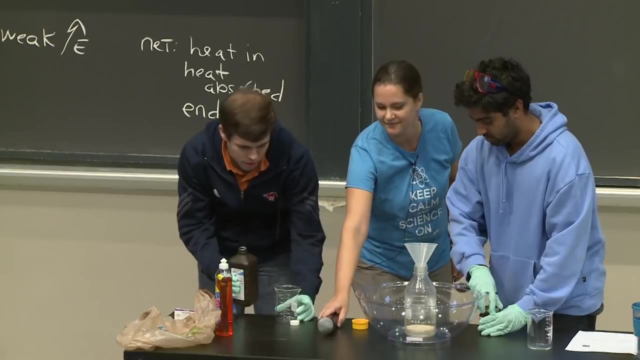 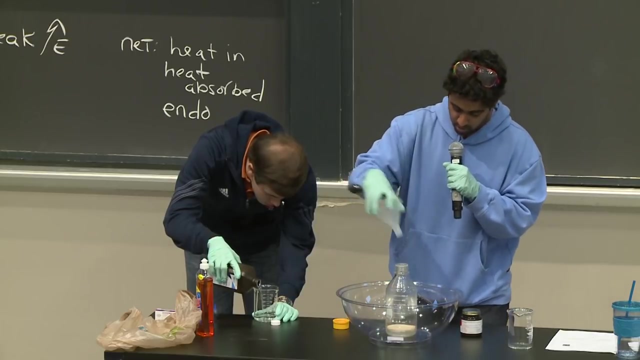 actually see disorder increase. If you want to just say, if you want to talk at the same time, here's a mic, It's on, Yes, it is Okay, great. So what we have going on here is: we've got this container. 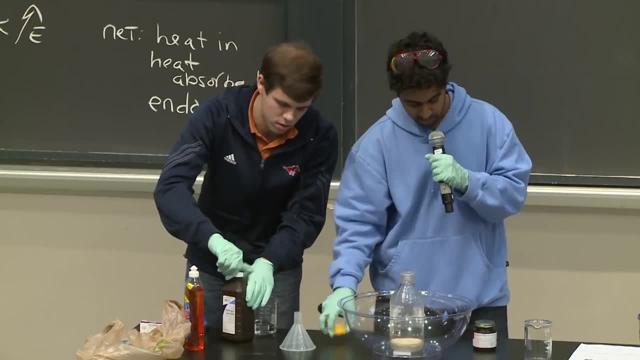 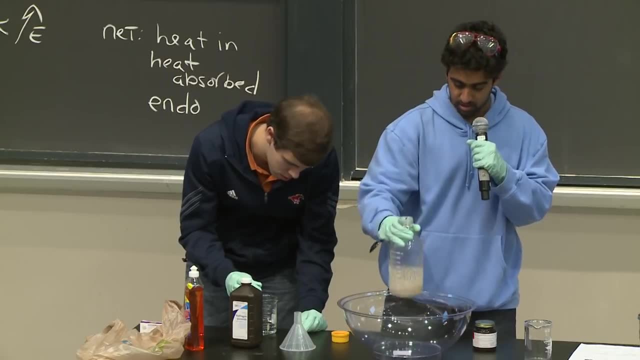 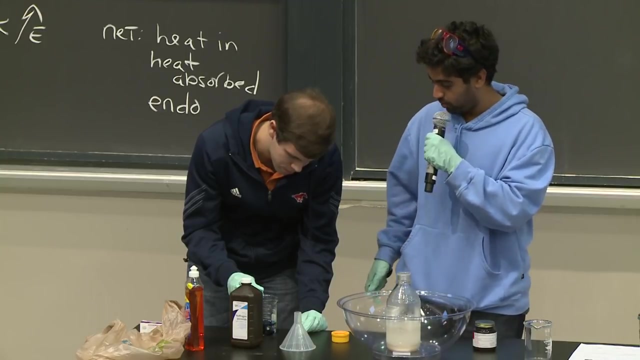 It's filled with water And what I did was I added about four teaspoons of yeast. The yeast, as Kathy said, is going to act as a catalyst. It's actually a biological species. It's actually going to, it's a living species that's actually going to catalyze this reaction. What, Eric? 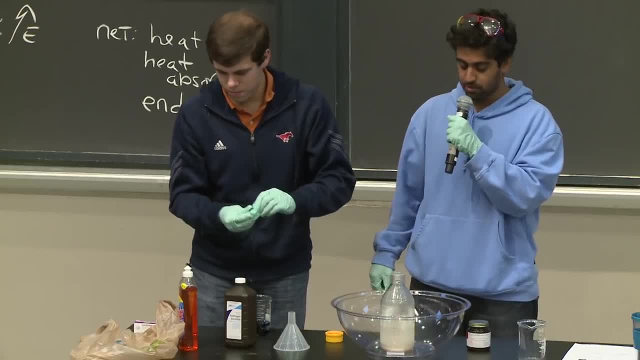 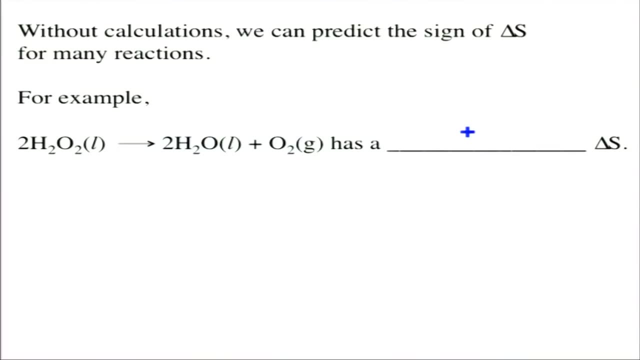 is doing is Eric is pouring some hydrogen peroxide. He added some soap. So, as you see, in the reaction the H2O2 is going to break down into water and gas, the gas being oxygen, And what we don't want to happen is we don't want just the gas to escape, because then you guys can't see it. So 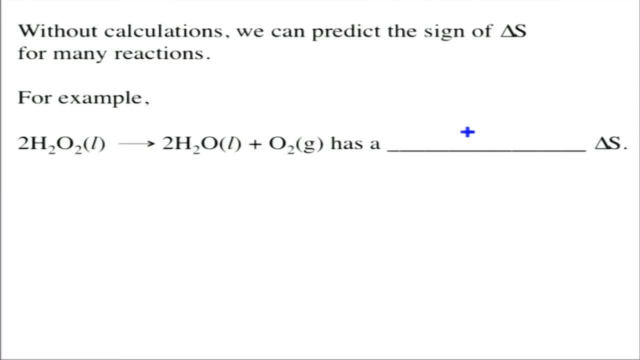 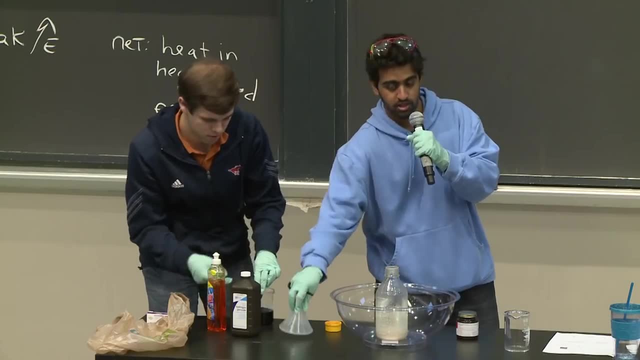 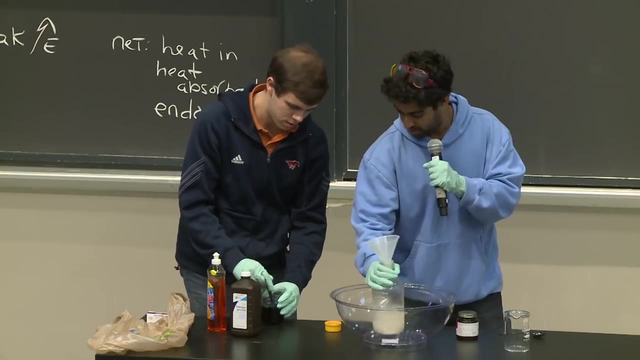 what Eric is doing right now is he's adding some soap. The soap is actually going to catch, if you will, the escaping gas and turn it into a foam, And what we should be able to see is the foam kind of escape from this container. You ready, Okay. so hopefully this will work. We should put on. 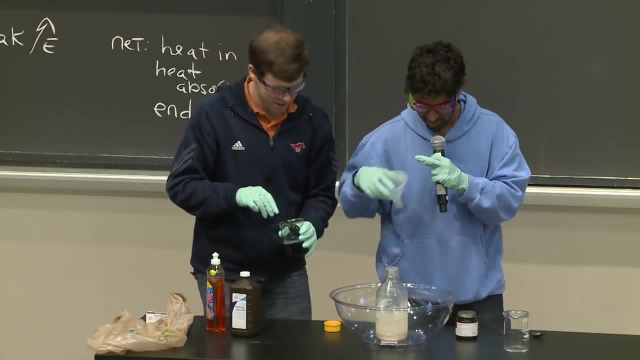 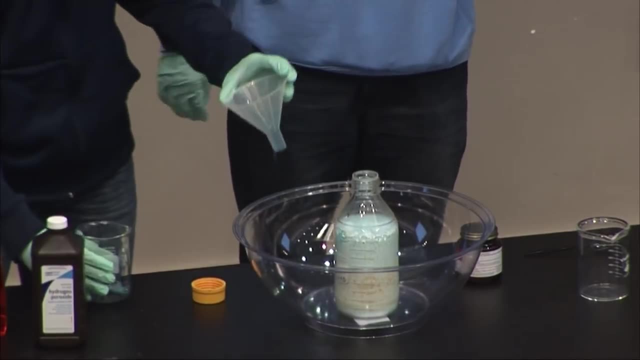 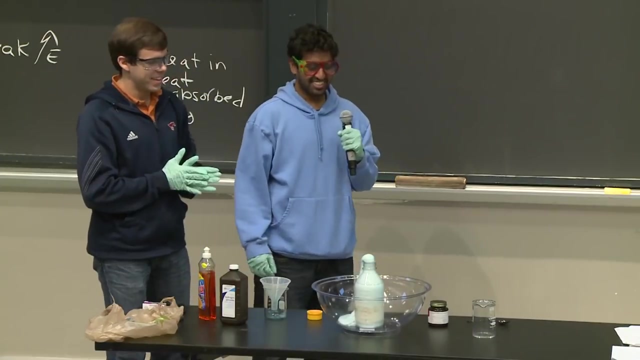 our goggles. It smells really bad. Okay, ready, All right, And get out of there. Look at that. Hey, wow, that worked a lot better than we thought it was going to work, And so this is something that's called the elephant toothpaste demo, because that is sort of what. 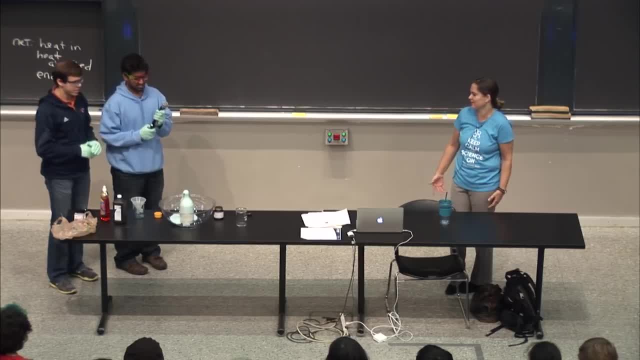 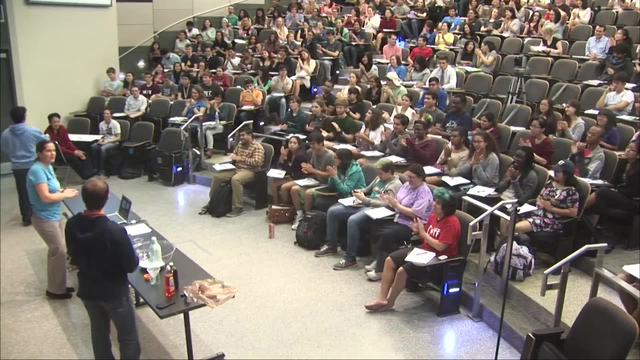 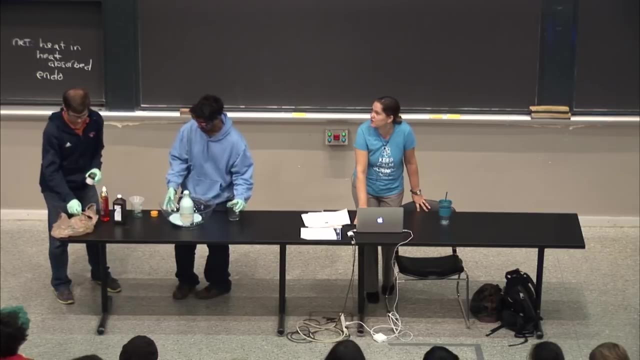 if you were an elephant, what you would probably be Brushing your teeth with, I don't know. Yes, So this is entropy increasing. Okay, so let's just see if we can quickly talk about a little more about entropy, and then we'll. 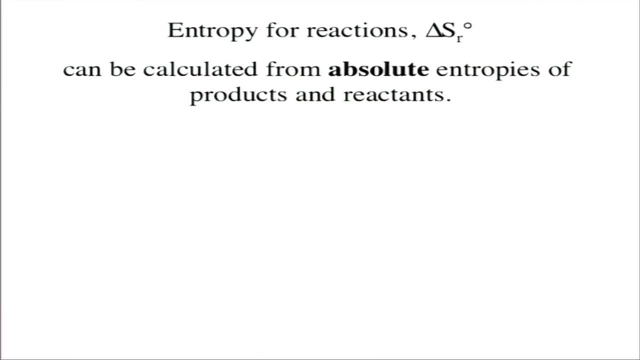 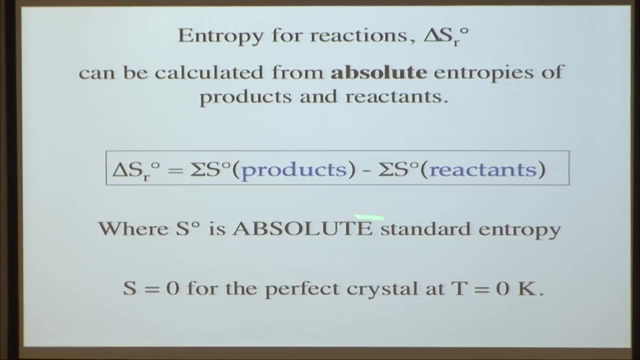 end. So entropy of reactions can be calculated from absolute values. And again we can use this equation equation here. So we have the delta S for a particular reaction. This can be calculated from the delta S's of the products minus reactants. So again we have products minus reactants. 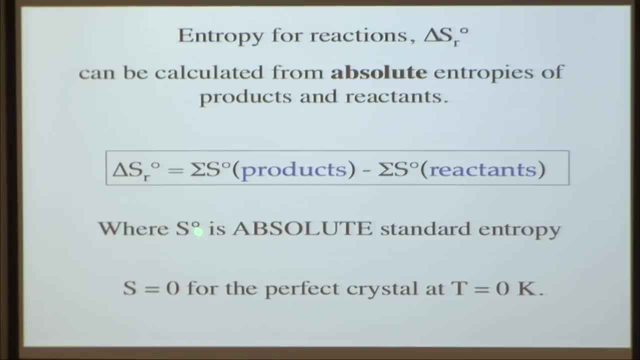 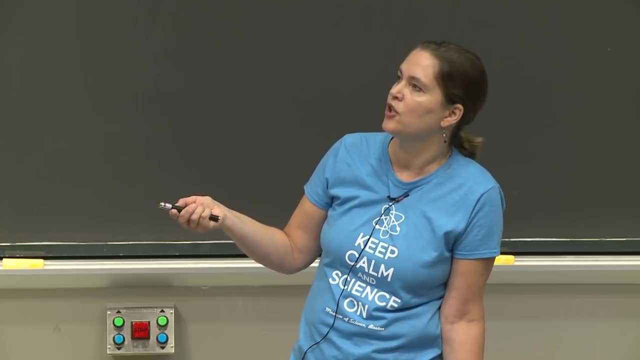 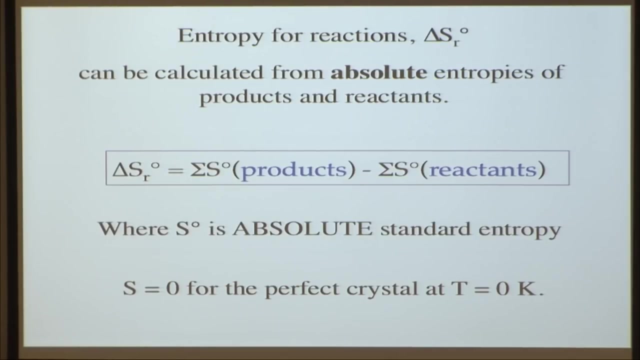 The absolute value or an absolute delta S. S equals 0 for a perfect crystal at a temperature of 0 Kelvin. You never really talk about S by itself. It's always really delta S And S of 0, this is like the saddest thing for a crystallographer, because you know you're. 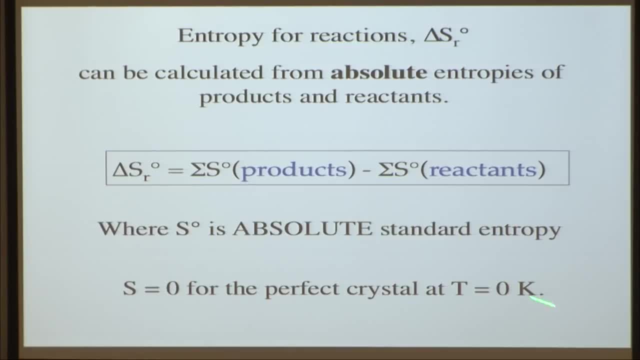 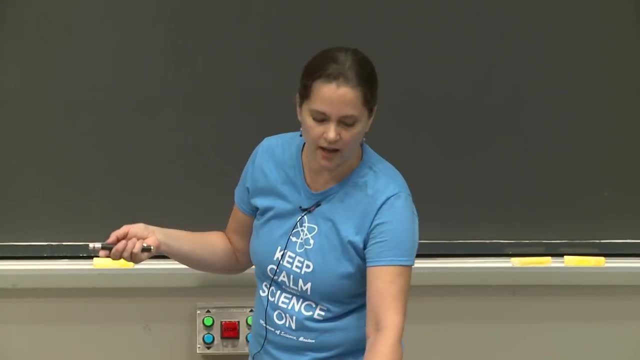 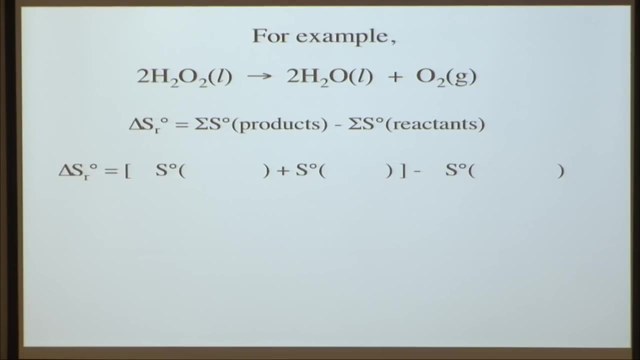 never going to have a perfect crystal, Even if you go to 0 Kelvin, I feel like, at least experimentally. So S equals 0, to me that's kind of sad. OK, So if we just put in for this reaction that we just did, we can put in our reaction. 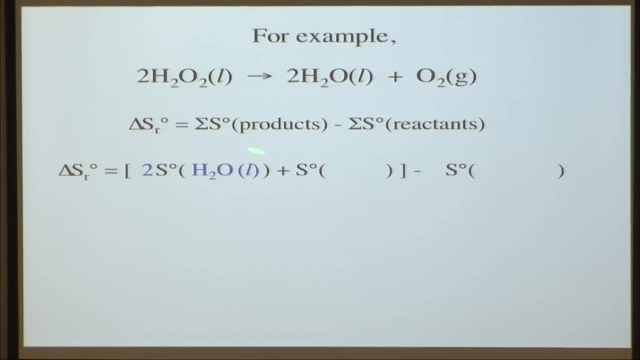 We can put in our values here And we can put in: we're forming liquid water and we're forming O2 gas And we are using two molecules of hydrogen peroxide, H2O2, here, And so now we can calculate what that delta S naught is, And it's a value of 125 joules per Kelvin. 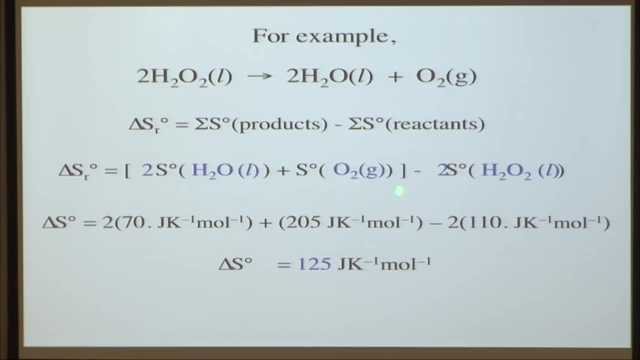 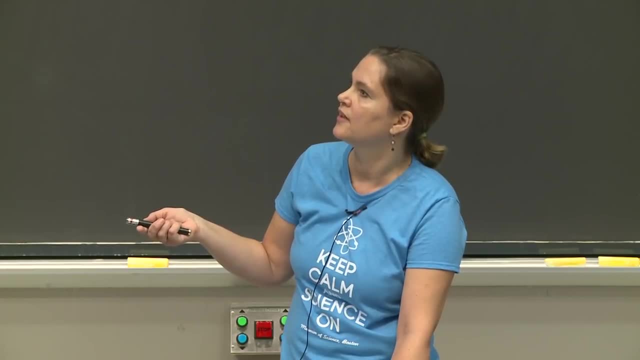 per mole. So again, products minus reactants And we can put in our values here And we can put in our units the numbers of products, water and gas minus reactants. Pay attention to the stok hagoe and you can get your delta S value. 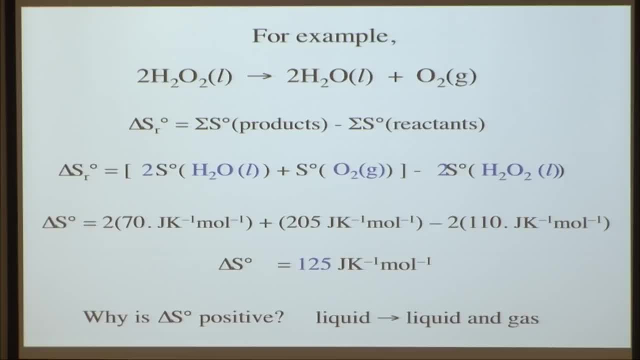 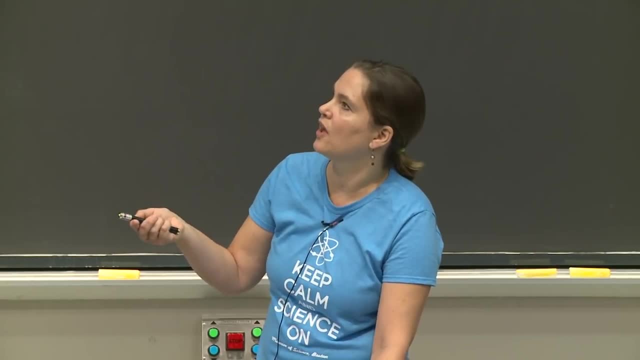 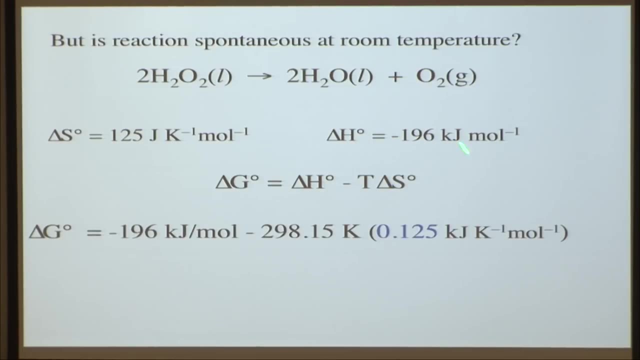 And why is it positive? Again, we already talked about this, Because it's going from liquid to a liquid plus a gas. And then, if we plug these values in again to see if it's spontaneous, we can use this equation and plug in our values, making sure we change. 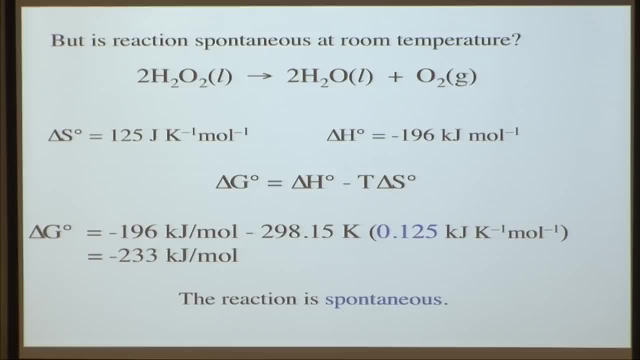 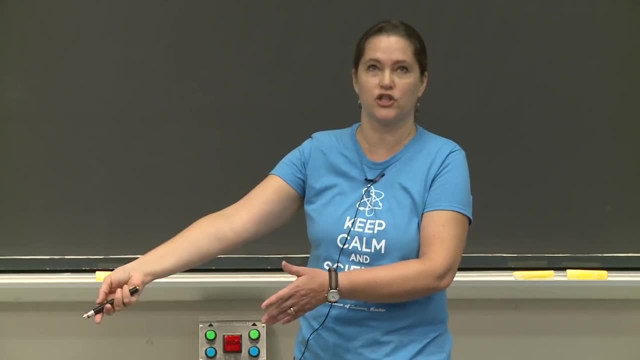 our used OK. So that's thetherma way that we sort of get to the delta S value here without units, and we can see that in fact this is a spontaneous reaction because it's negative here. but you already knew that because you watched it go spontaneously. 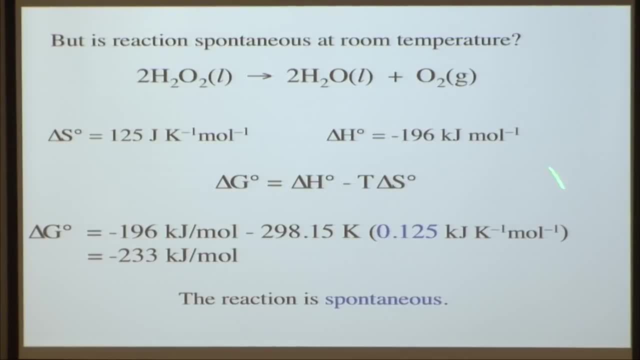 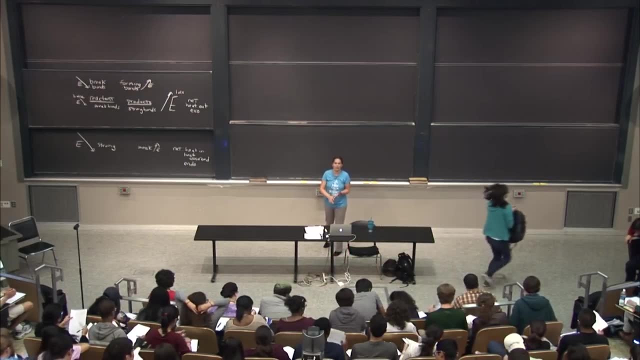 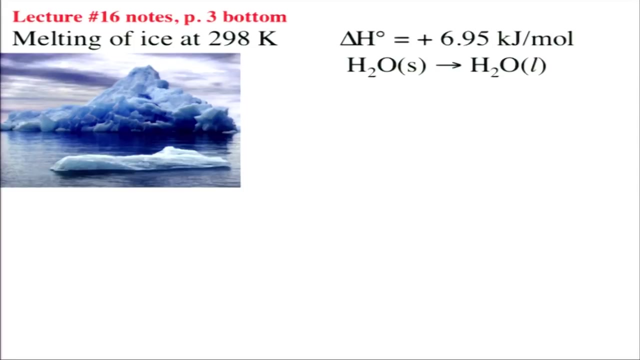 So most of the time you can't do the demo, so then you can use this awesome equation right here, OK, So that's where we're stopping for today and we'll see you all on Friday, All right? So if you take out your lecture, 16 notes on the bottom of page 3, we had an example. 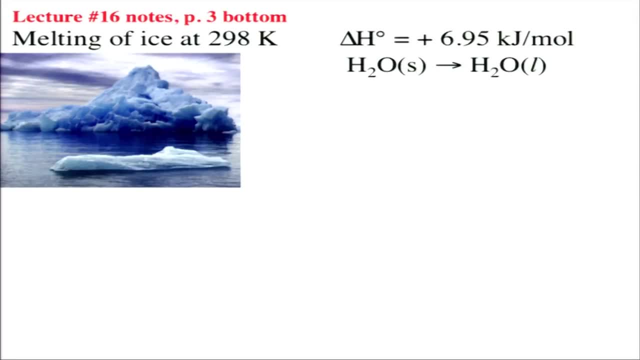 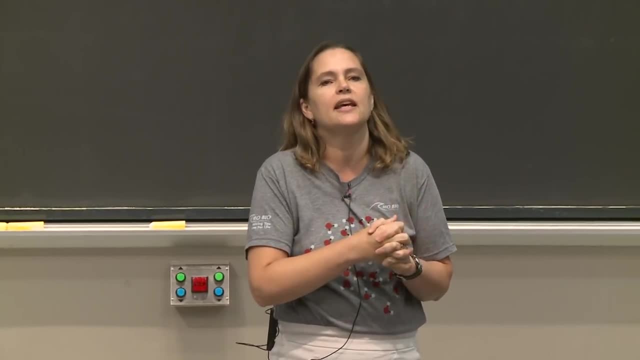 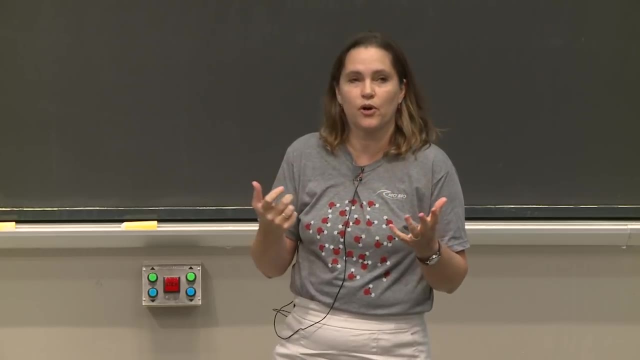 about the melting of ice at room temperature. So we did a little demo for you at the end of class last time and calculated that the reaction was spontaneous for hydrogen. Hydrogen peroxide is pretty reactive and we watched the O2 bubbles go and we did that. 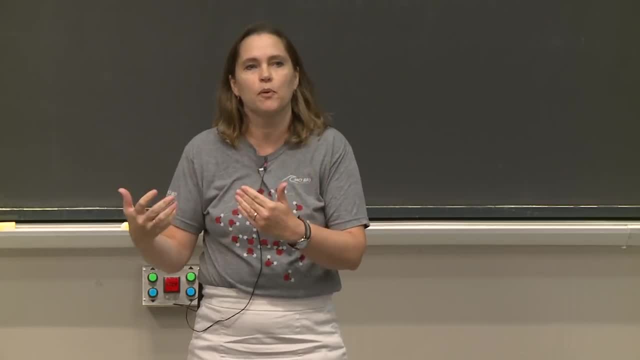 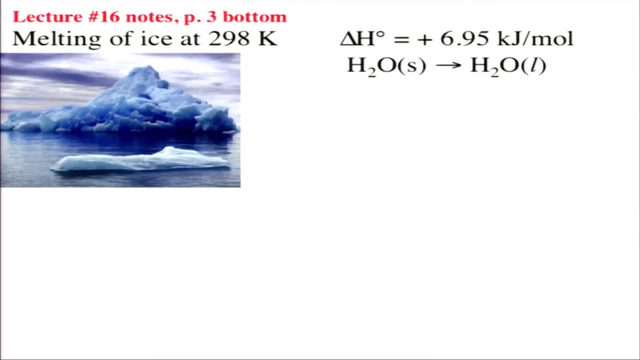 calculation. So we're thinking about not just delta H, but we're thinking about delta S and we're now thinking about delta G as well and how they all play together. So when we started last lecture, we had talked about the fact of some reactions that were 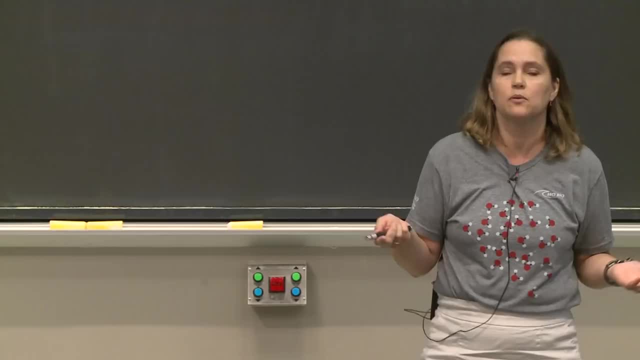 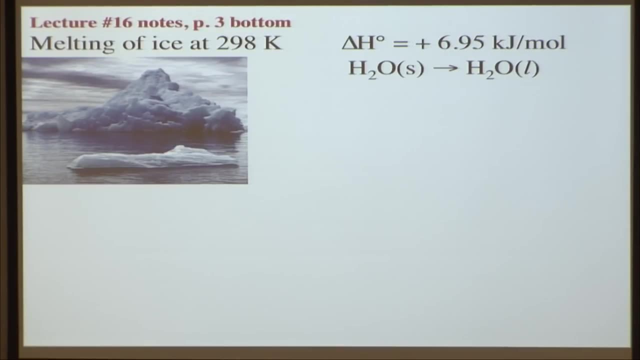 spontaneous, where delta H was negative, where it was exothermic, where heat was released. But then we also gave some examples where delta H was positive and said: but these are also spontaneous reactions. We all know that at room temperature ice will melt. 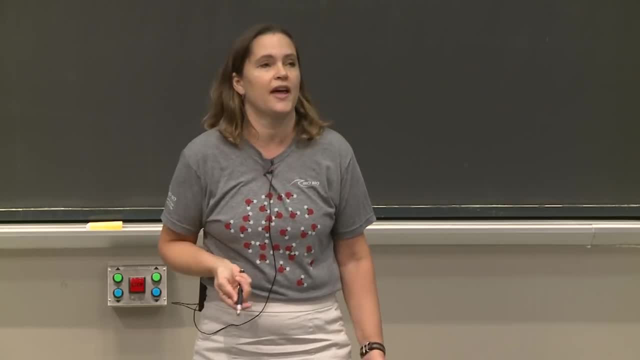 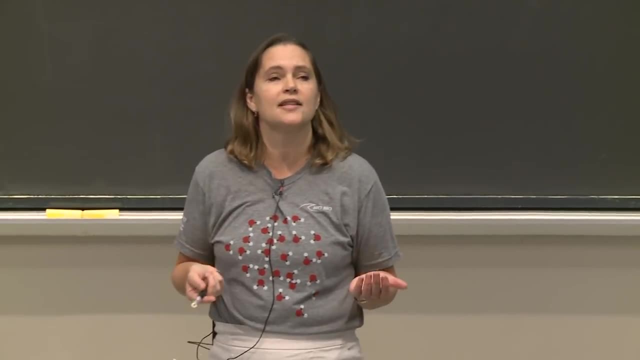 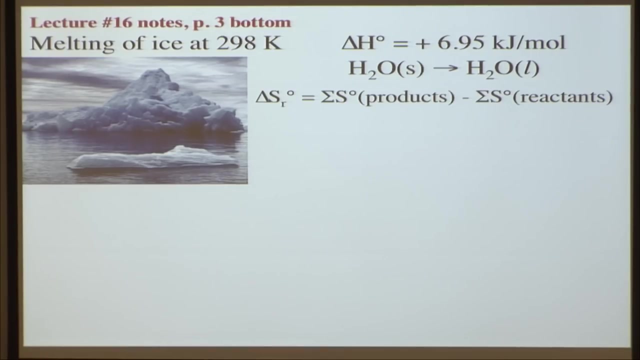 We know that that's a spontaneous reaction, But the delta H for that reaction is actually a positive value. It's an endothermic reaction. So when we're thinking about these reactions in spontaneity, we have to be thinking about delta G, not just delta H, And delta G has to do with delta H and delta S. So sometimes 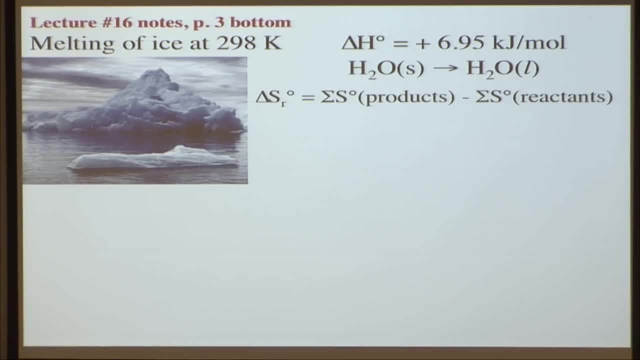 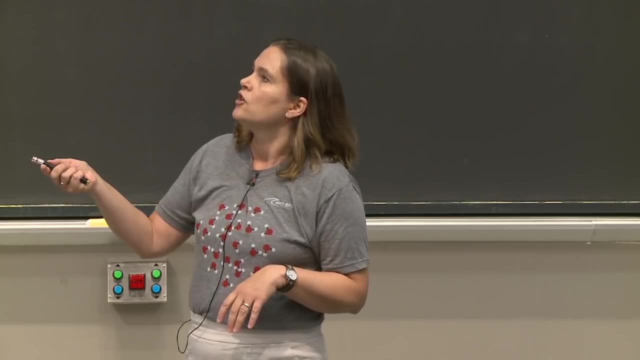 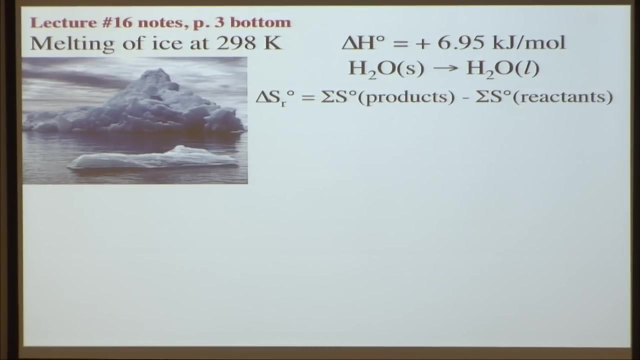 delta S is the driving force behind whether a reaction is going to be spontaneous, whether the delta G will be negative or positive, Delta S is making that determination. OK, So we can calculate what a delta S for a reaction is if we know the entropy values for the products. 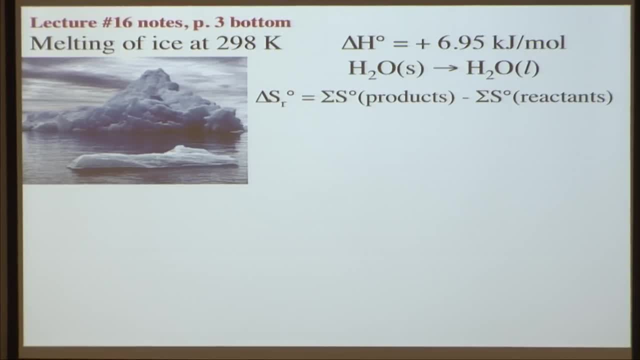 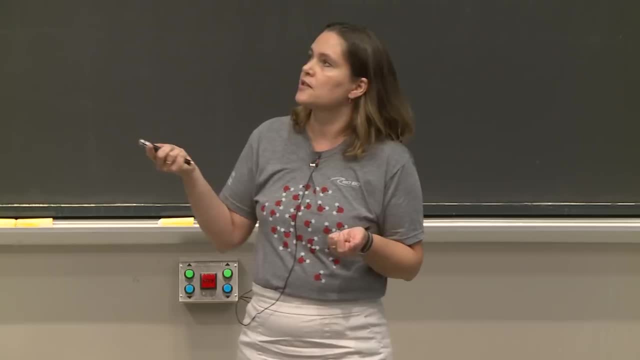 And it's the sum of the entropy values for the products minus the sum for the reactants. So when we are doing heats of formation, we also have products minus reactants. But we have one exception to this- products minus reactant rules- And that's when we're using what. 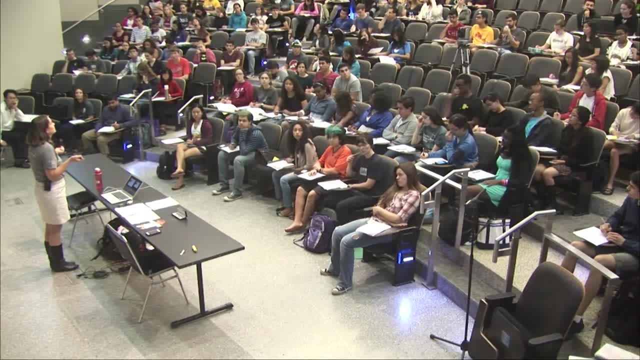 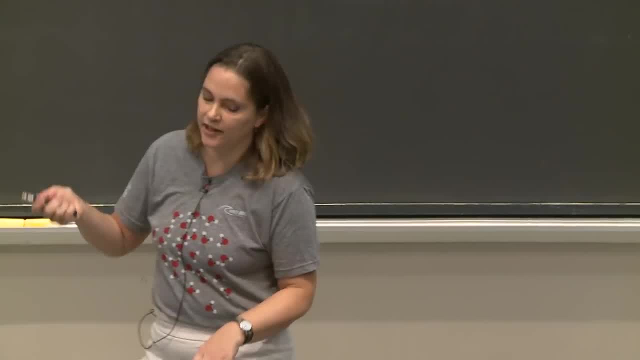 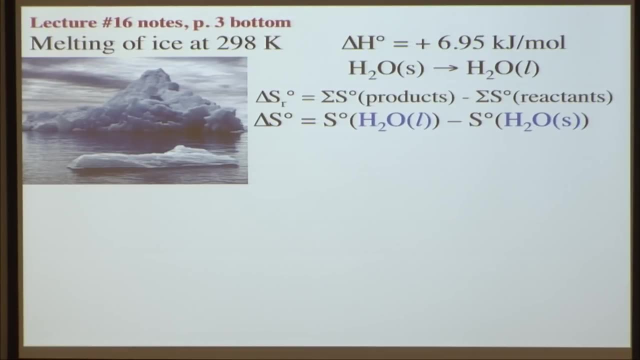 What thing are we going to do? reactants minus products, Bond Bond, Envelopes, Envelopes, Right, OK, But here we're: products minus reactants, So we can plug those numbers in Our product is our liquid water. 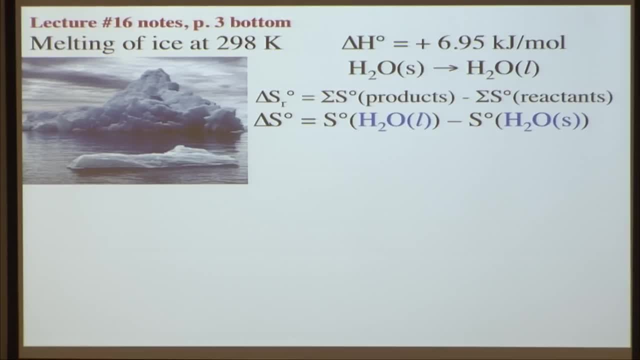 Our reactant is our solid water or our ice, And we can calculate what the delta S0 is for this reaction. We can put in our values And we get a positive value, Positive 28.59.. OK, OK, Thanks. 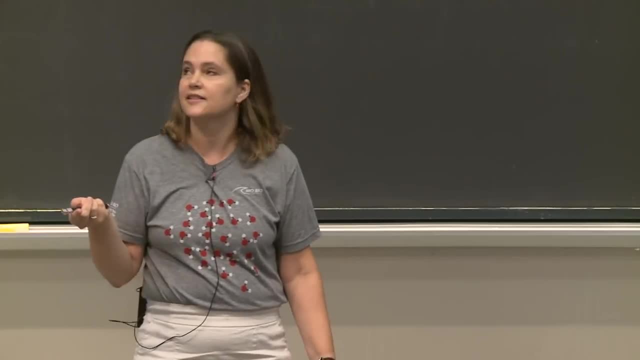 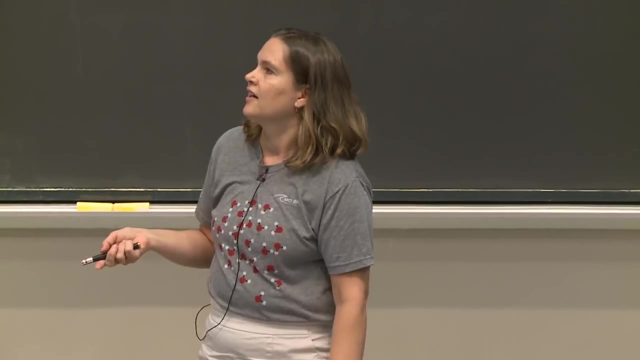 Amazing. Well, see, see, I always remember this. Delta S0 times 6したs tends to be u in joules per kelvin per mole, And delta Ss tend to be in joules. Everything else is in killa joules. 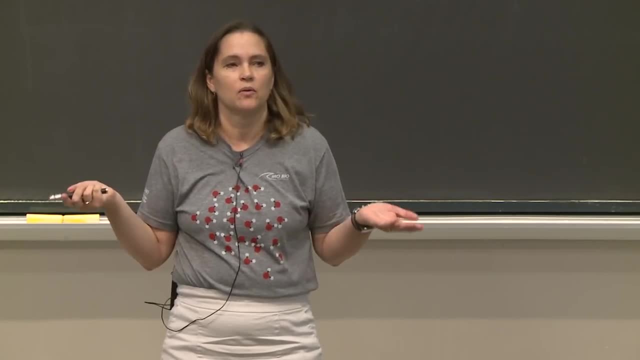 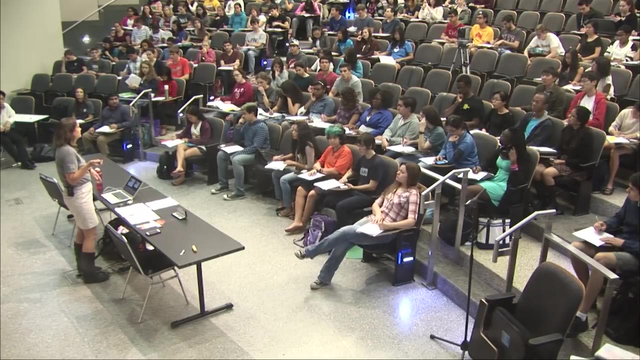 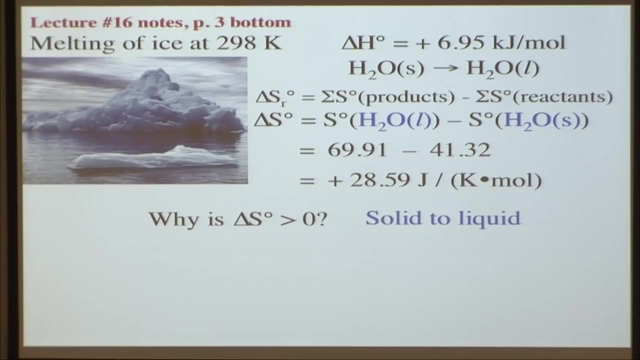 So keep that in mind. And why do you think this reaction? it has a positive value? Why is delta S greater than zero? Yeah, so we're going from a solid to a liquid, So we're increasing the internal degrees of freedom. 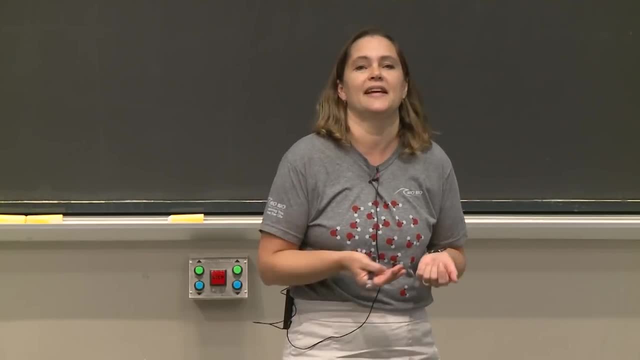 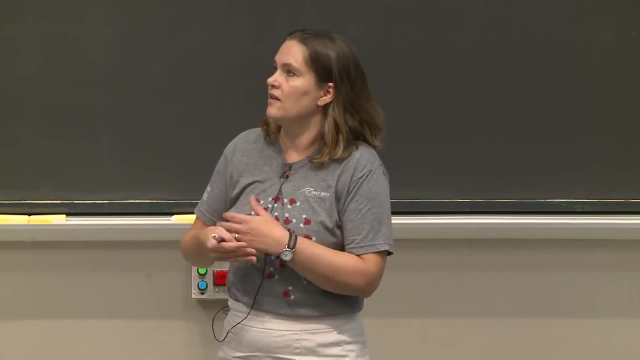 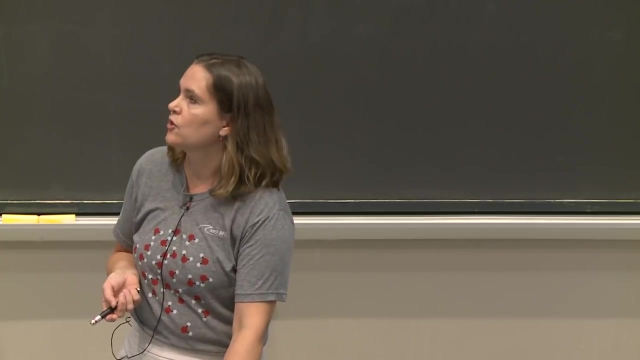 The molecules of water can move around more in a liquid than they can in a solid. So this is increasing the disorder of the system, increasing entropy here. because the water molecules can move around more, There's more freedom of motion. So delta S is positive. it's increasing. 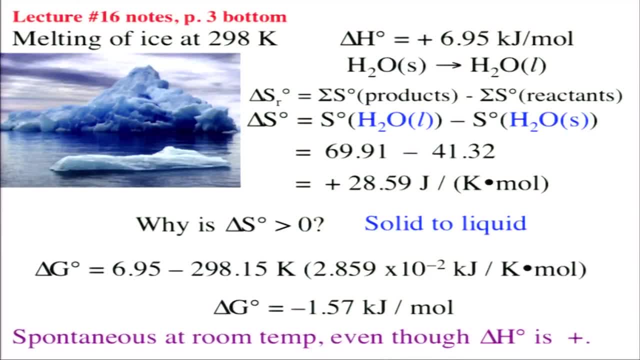 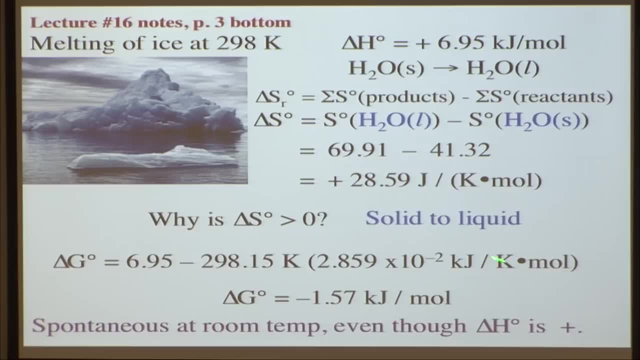 And then we can use that to calculate delta G: naught gives free energy. We can plug in our delta H value minus T, room temperature times. delta S, which we just calculated, making sure that we convert from joules to kilojoules. 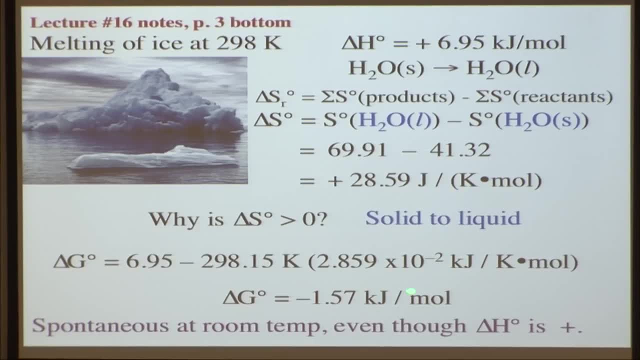 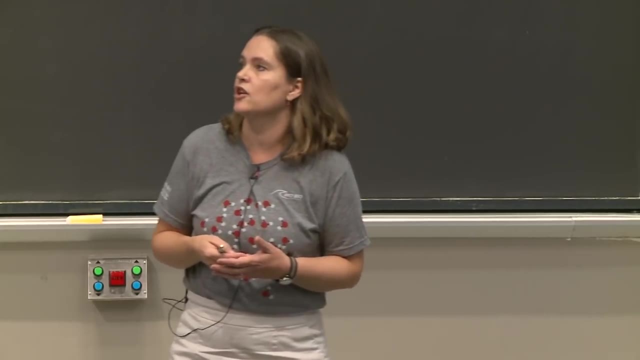 And then our units will be kilojoules per mole, And here delta G naught is a negative value. So it is spontaneous. We all know it's spontaneous, We've observed this happening. So even though delta H naught is positive, it's an endothermic reaction. ice melts at 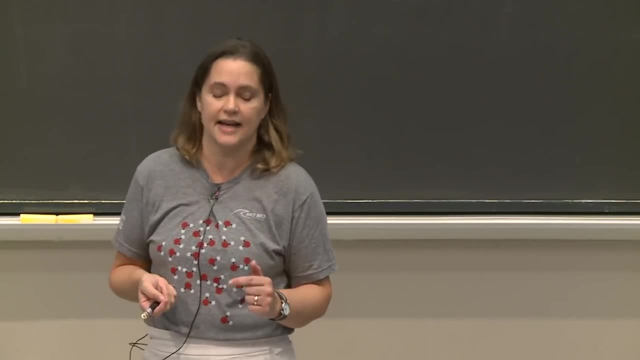 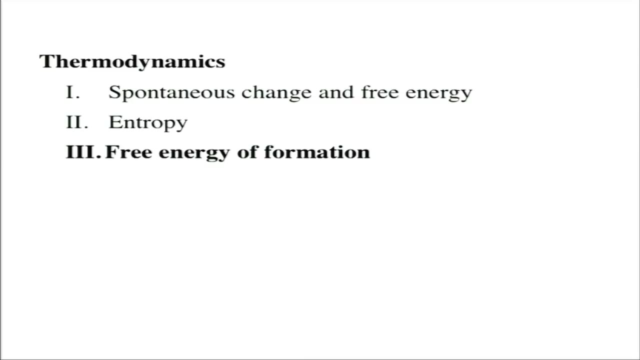 room temperature because the delta G is negative. All right, so let's talk a little more about delta G. So let's talk about free energy of formation And the last page of this handout, so free energy of formation, delta G, sub F, And so 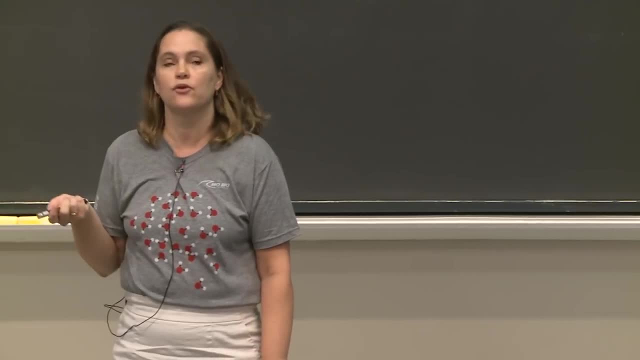 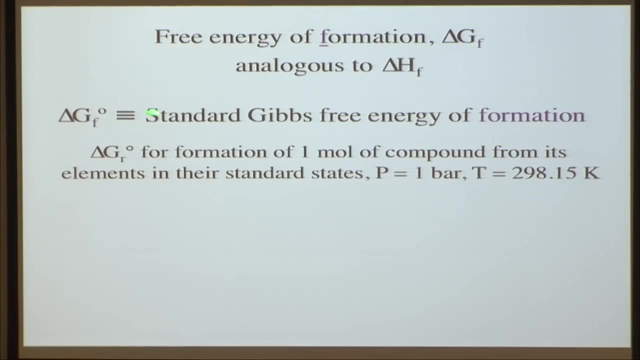 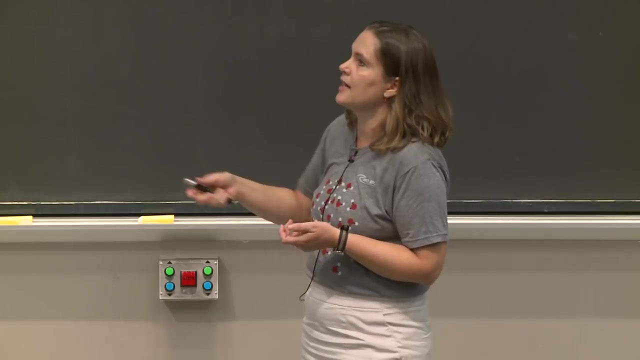 this is analogous to delta H of formation, so the change in enthalpy of formation. So again, when you have the little value here, the standard gives free energy of formation for the F here, And that's the formation of one mole, of a molecule, from its elements in the most stable. 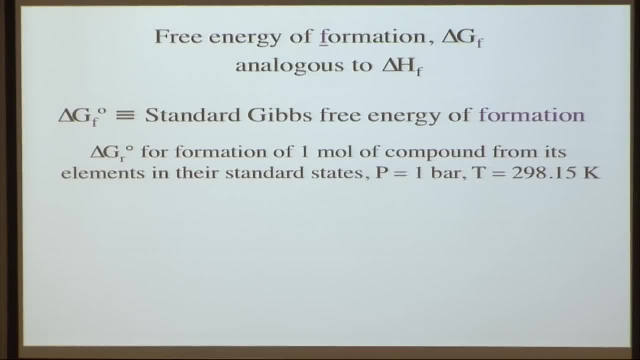 state and in their standard states. So we can have tables. We have tables in your book of these values. So your book in the back- if you haven't explored the back of your book- there's lots of tables of things, including information about delta Gs and delta Hs and bond enthalpies and all. 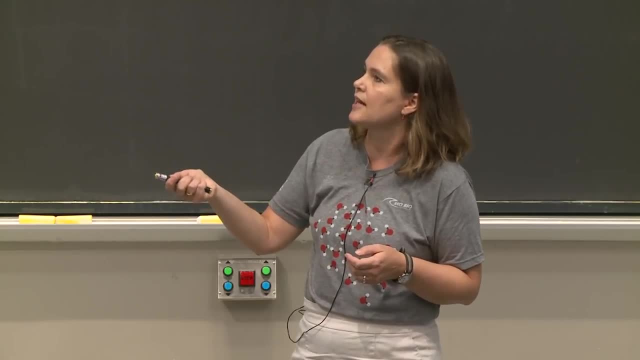 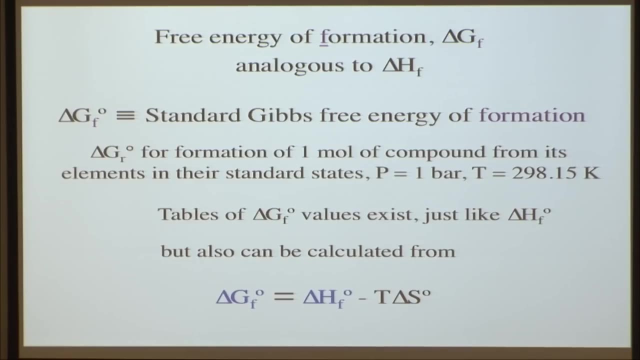 sorts of other things, redox, potentials, we haven't talked about yet lots of tables, So you can look this up. Or if you have already say, looked up your delta H of formation, you can use this handy equation: Delta G equals delta H minus T, delta S. But if we plug in our delta Hs of formation, we 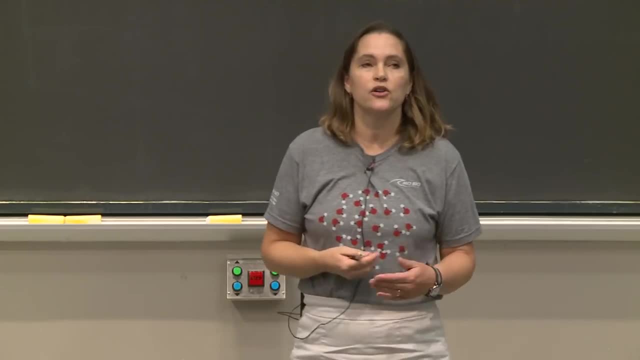 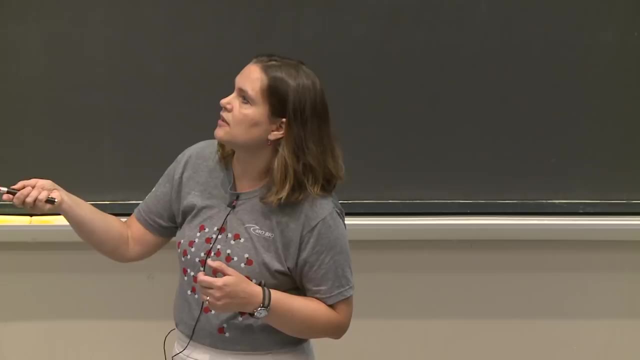 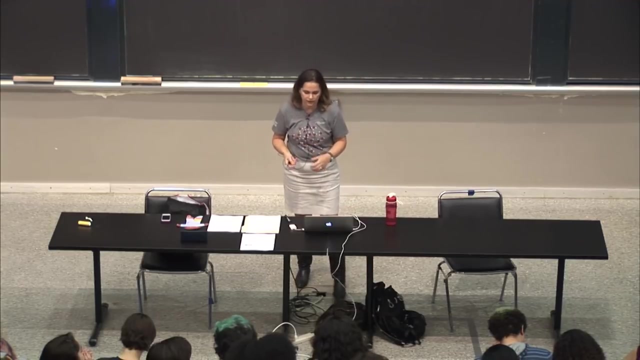 can get our delta Gs of formation. So how you're going to calculate delta G of formation depends on what information you are given. So let's think a little bit about what it means for particular delta Gs of formation if they're positive or if they're negative. 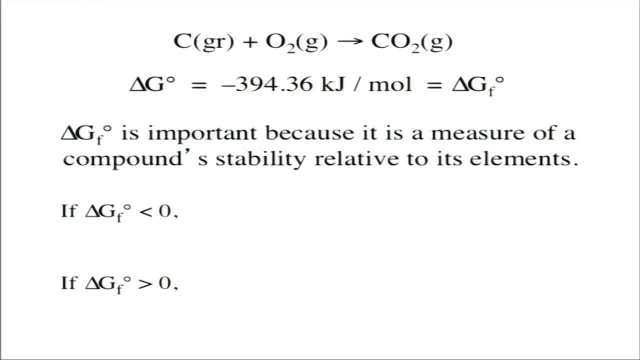 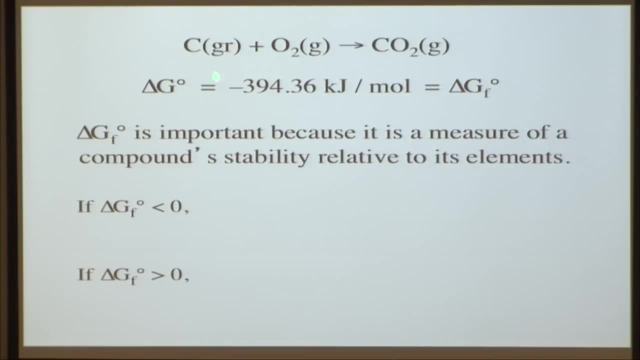 So let's look at an example. We saw this before. This is the formation of carbon dioxide from elements in its most stable state, which is graphite, carbon and O2 gas. So these are the elements in their most stable state forming CO2.. 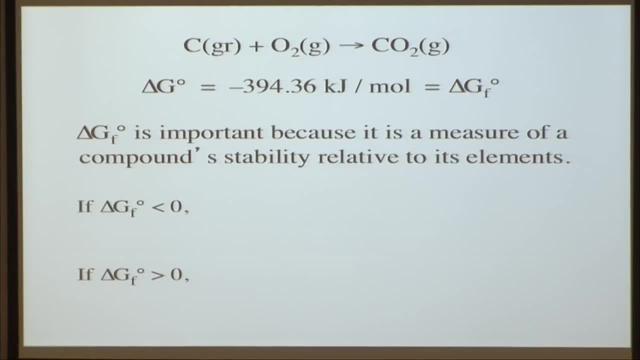 Now I'm telling you that the delta G naught is minus 394.36 kilojoules per mole, And we can think about what this information tells us, that this is a fairly large negative number. So it depends on where you plug in the gamma ion inside. 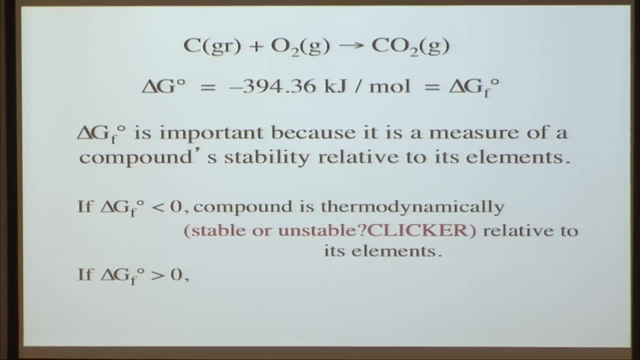 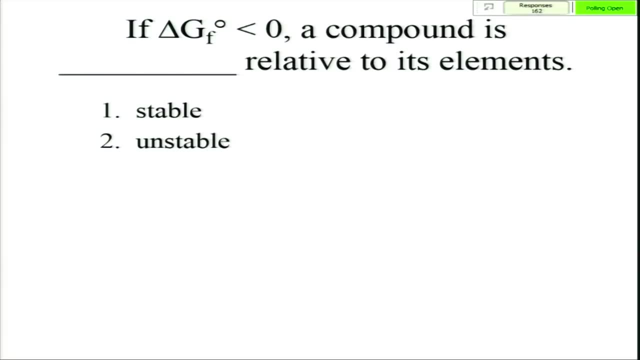 So if delta G of formation is less than zero, what's going to be true thermodynamically- And this is a clicker question Which umpire is the polarities between mass prime and mass prime. This is a списикс indicator. 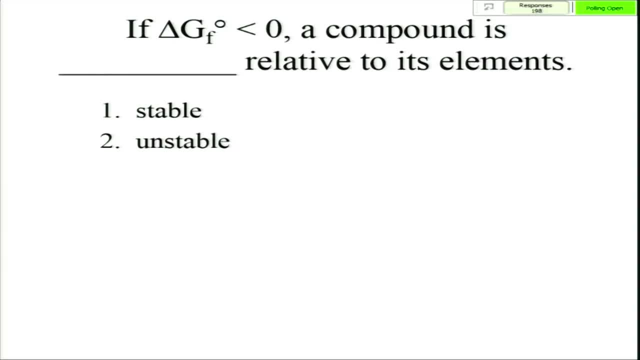 This is kind of like partol and黄. This is more or less an☆. This is an equation. You've got it right. Yeah, You've got it All right. let's just take 10 more seconds Interesting, okay. 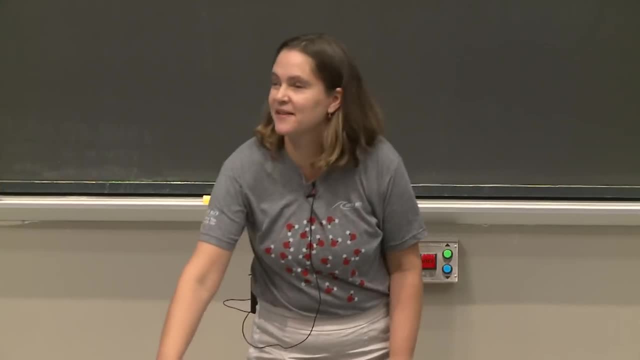 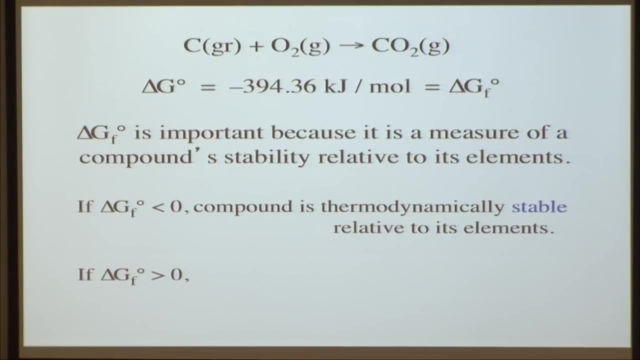 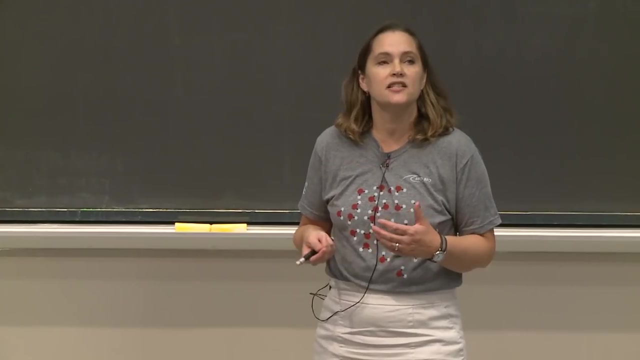 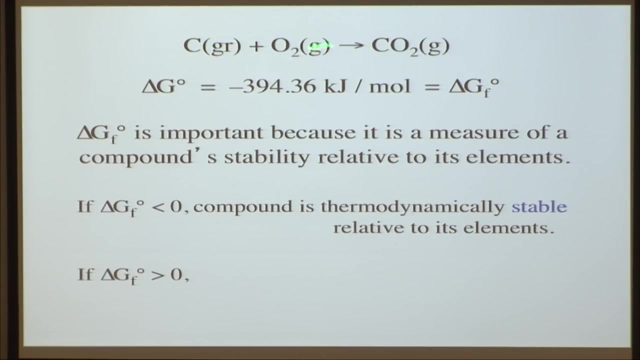 So let's think about why this is true. This might be a deciding clicker question, we'll see. So if it is negative value for delta G, a negative value for delta G means that it's spontaneous in its forward direction. So here the formation from the elements in their most stable state. if this is spontaneous, 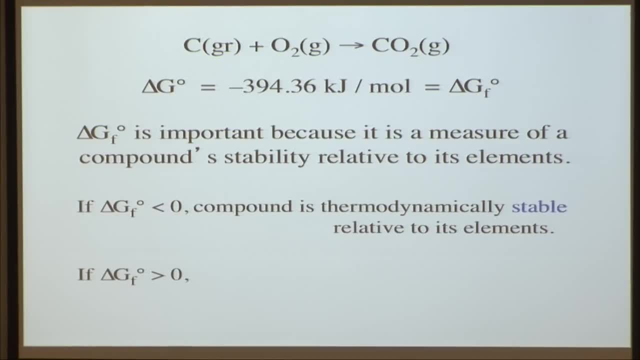 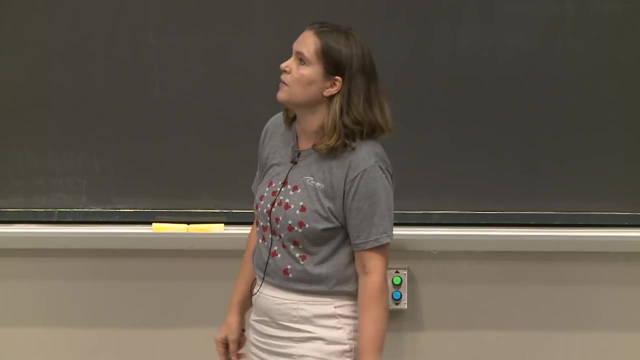 in the forward direction. it also means that it's non-spontaneous in the reverse direction. That means one CO2.. It's going to be stable compared to the elements from which it came because it's non-spontaneous going in the reverse direction, or at least that's the way that I like to think about. 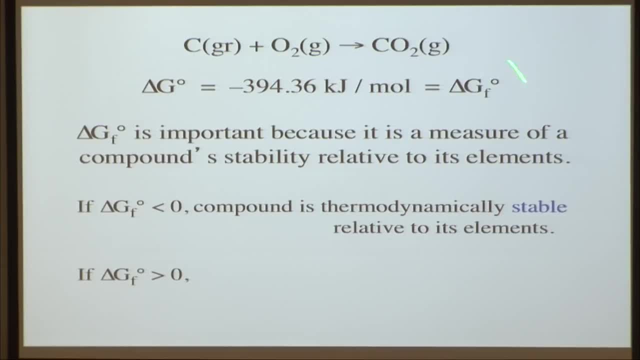 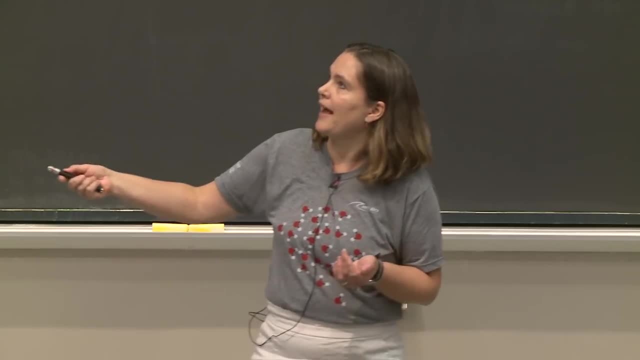 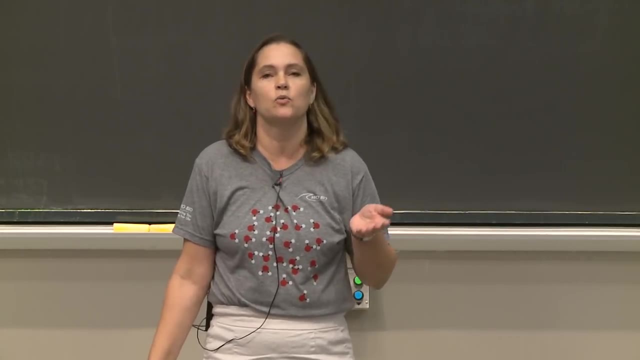 it. So, relative to its elements, it's stable, Spontaneous forward, non-spontaneous in reverse. So this is kind of bad news for us, because there's too much CO2 in our environment right now. It's a greenhouse gas. And wouldn't it be awesome if we could just encourage it all to go back to its elements for more oxygen which we could breathe. How lovely. make some nice graphite, maybe compress it, make some diamonds. but no, It is quite stable compared to its elements. 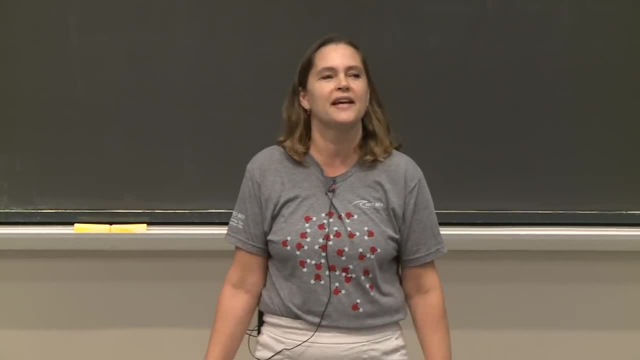 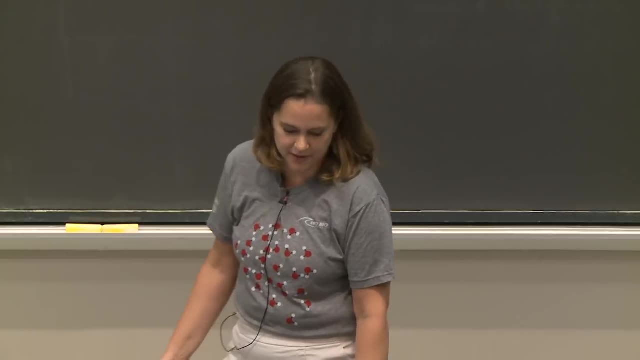 So CO2 is in our environment, causing global warming, and it's going to be hard to solve that problem, not easy to solve that problem. So this is unfortunate news that thermodynamics gives us All right. So then we can look at the other. 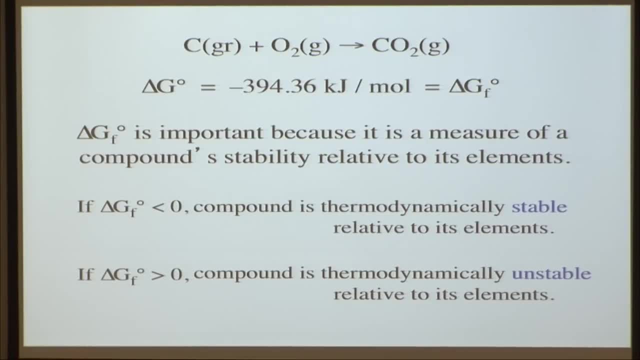 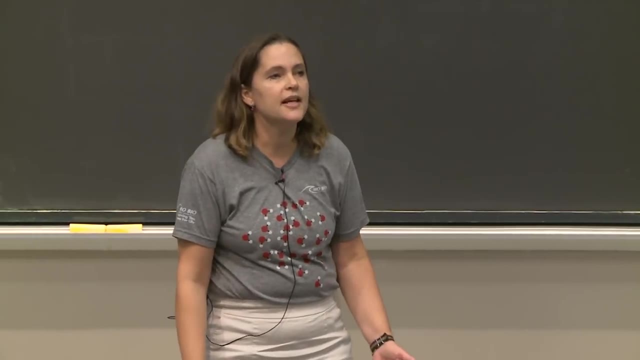 If you have a positive value for delta G of formation, then it's thermodynamically unstable compared to its elements, So it's spontaneous going in the reverse direction. so it's unstable. So thermodynamics tells us whether something is stable or unstable and kinetics tells. 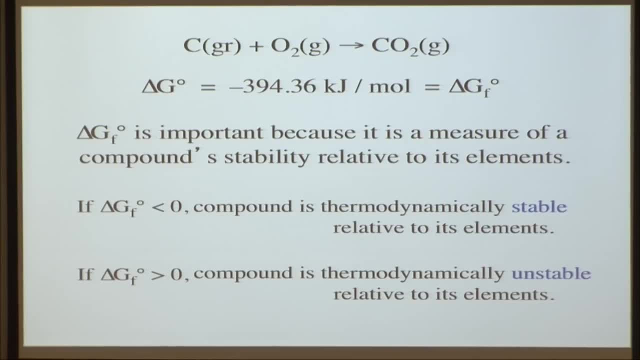 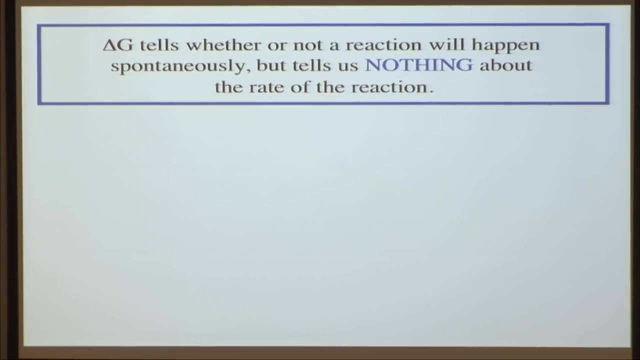 us about whether things will react quickly or not. So something can be kinetically inert, It might take a long time to react, But thermodynamics tells us: stable, unstable. So thermodynamics is great, but it doesn't tell us anything about the rates of reactions. 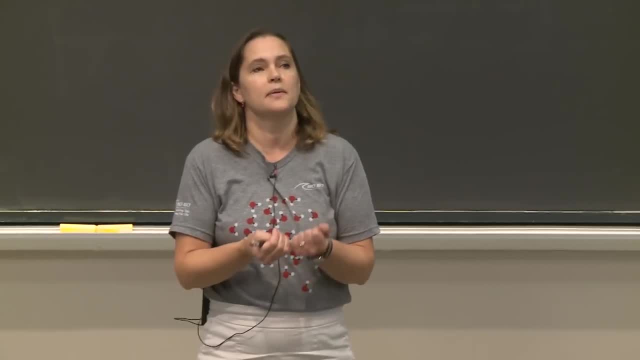 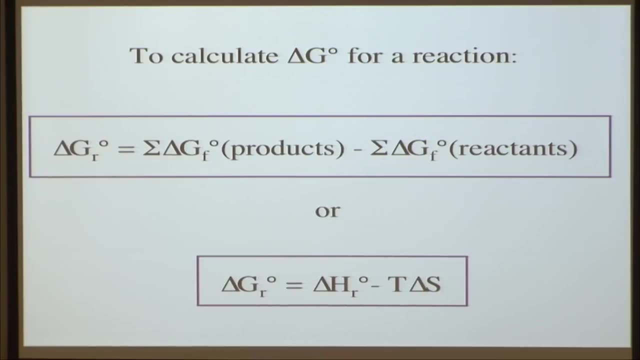 So nothing about the rates and that's kinetics. So really, thermodynamics and kinetics are very important for explaining reactions, And we'll talk about more kinetics at the end. So to calculate a delta G for a reaction, It doesn't take a lot of time.